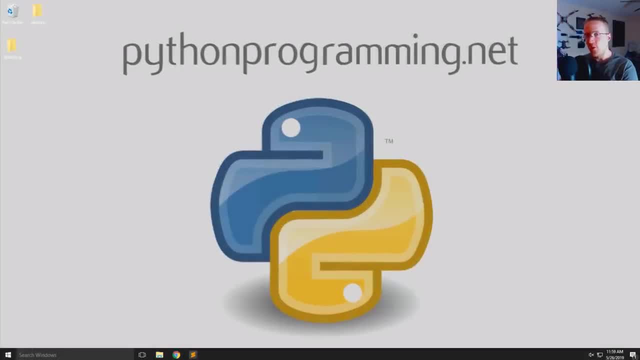 What is going on, everybody, and welcome to a reinforcement learning tutorial series. In this video we're going to be starting off with Q learning Now. every time I do a new series, people are like: what are the prerequisites Really for any of the series? there aren't any, Just anytime. 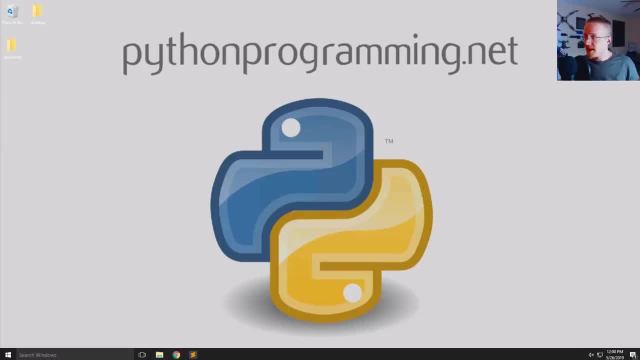 we hit a concept or topic you don't understand, look it up. In this case, though, there really shouldn't be anything. If you know basic Python, you should be able to follow along with the Q learning tutorials pretty well. Now, when we start getting into deep Q learning, that changes Now. 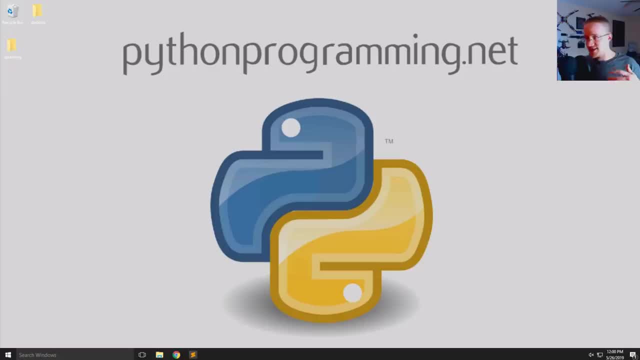 you need to know TensorFlow and Keras and stuff. So just keep that in mind. But at least to start, pretty much anybody should be able to follow along here. So first of all, what actually is Q learning? The idea of Q learning is to have these like Q values for every action you could possibly. 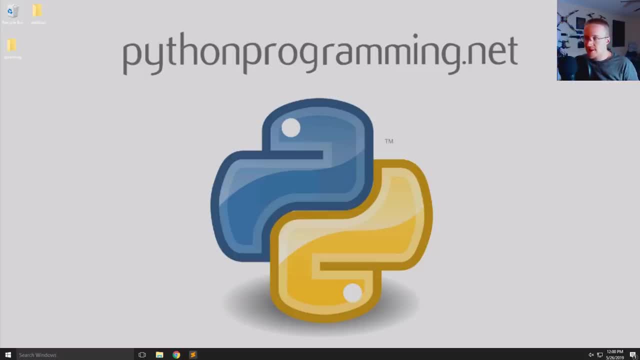 take, given a state, And over time we want to be able to update those Q values in such a way that running through a chain of actions will produce a good result. Okay, now that's done by rewarding some sort of agent as they get through this environment, And the idea is to kind of reward for the long-term goal, rather. 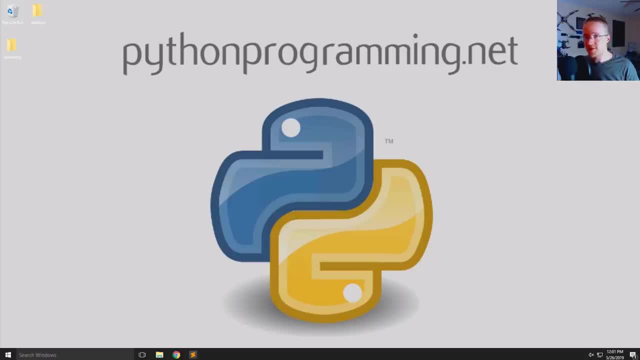 than in any immediate short-term actions. Now, Q learning specifically is what's called model free learning. The idea is that the Q learning model that we rewrite, basically the Q learning algorithm, is applicable to like any environment. It's not really environment specific, So the code that we write should be mostly 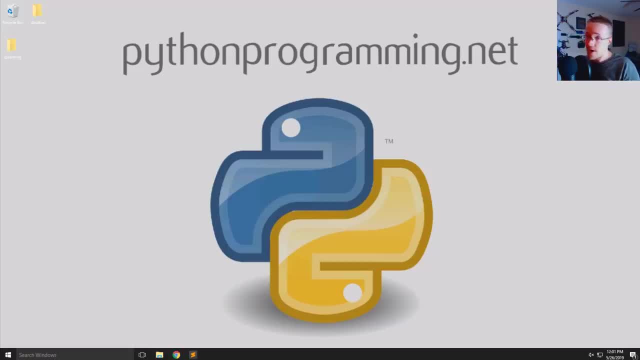 applicable to any other environment that we might want to use it in, As long as that environment's simple enough. So Q learning in the way that you know what we're about to work with is good for really basic environments, but it's not going to do anything really complicated. 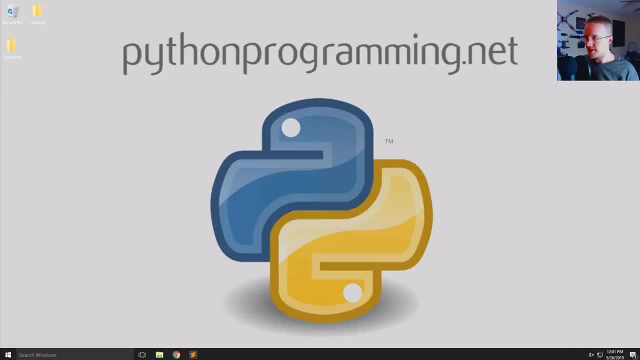 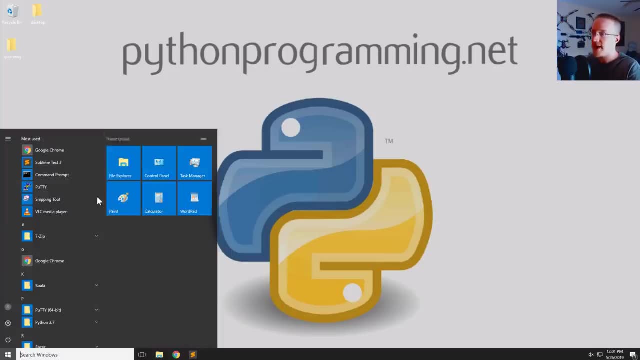 For that you're going to have to start getting into deep Q learning or something like that. Anyways, I think the best way to learn is by doing So. let's jump in. So we're going to need a couple of things right out of the gate. 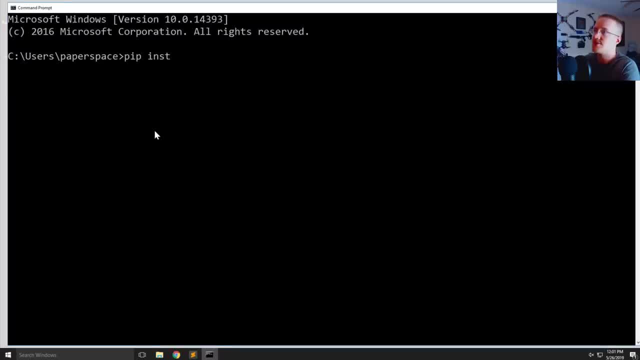 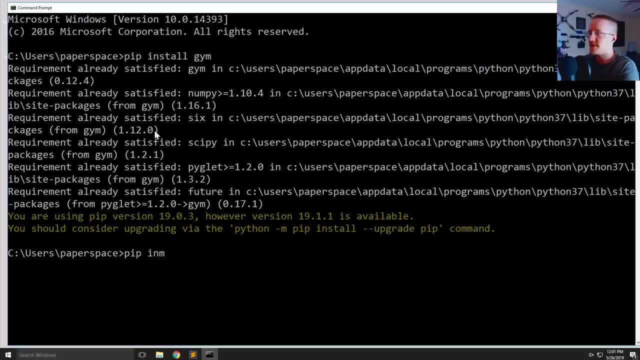 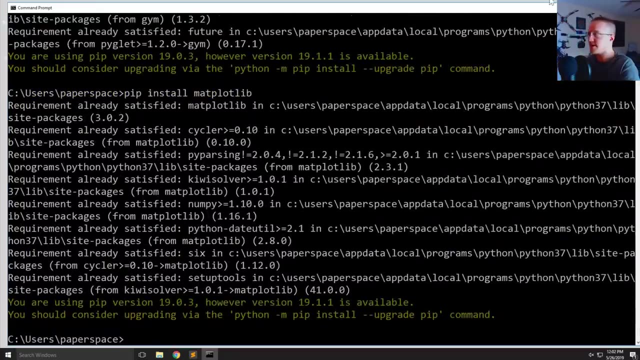 So go ahead and pip install, Jim, I should already have it. And then also go ahead and pip install if you can type. unlike me, install Matt plot lib. Grab that as well. We're going to be using that in a series and I might forget to tell you to get it. 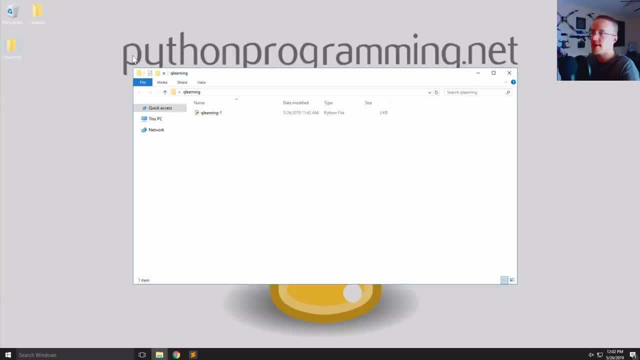 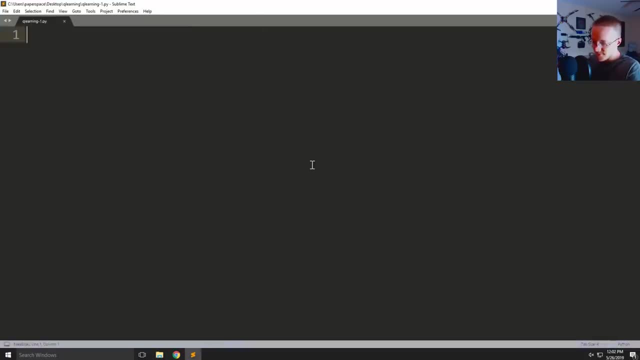 but that should be it. So I'm gonna go ahead and go into Q-Learning here and just edit. this file should be empty for now. Don't need that right now, Cool, So the first thing we're gonna do is just kind of poke. 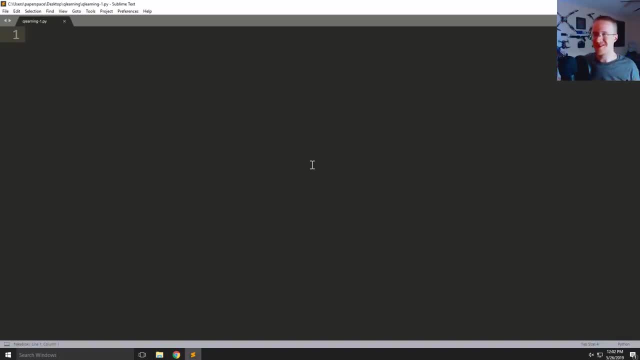 around get an idea for this environment. So, even though this environment doesn't matter much to our AI, it matters to you to understand how Q-Learning actually works. So what I'm gonna go ahead and do is fix this first of all. 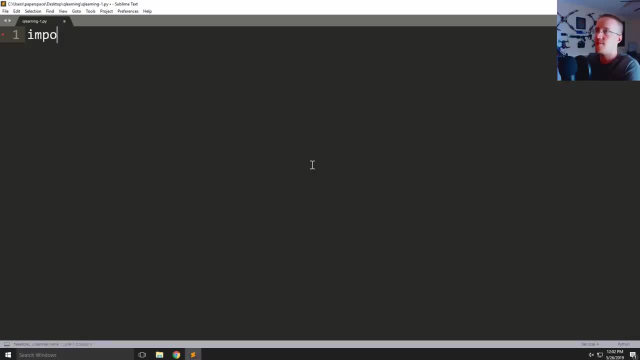 There we go, Import, import gym. and then what we're gonna say is: the environment is a gymmake, and the environment we're gonna use here is MountainCar-V0, and that's title case: MountainCar, Anytime you have an environment. 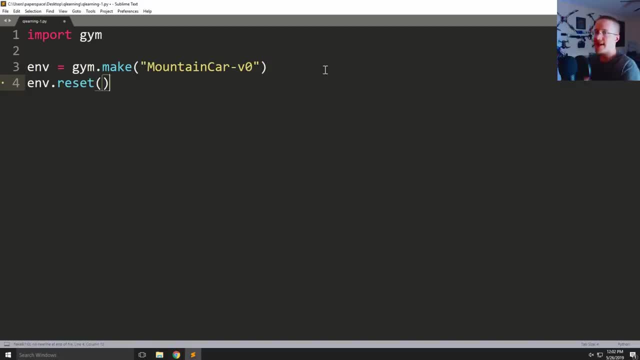 the first thing we're gonna do is reset, and then we are ready to actually iterate through this environment. So what we're gonna say is done equals false, and then, while not done, we want to step through this environment. Now. to do a step, we need an action. 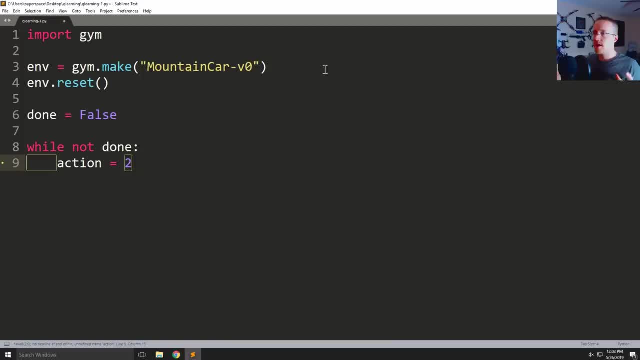 So for now I'm gonna say: action equals two. Now again, for your benefit. I think it's useful to understand how the environment works, but in terms of your agent, it doesn't need to actually know. But for your own information, MountainCar. 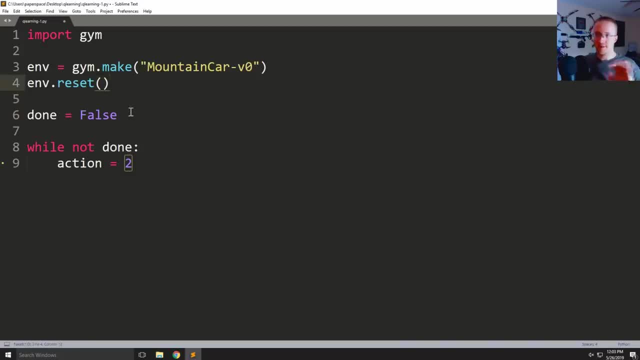 this environment has three actions that you can do: MountainCar- yes, take now in a little bit, i'll show you. you can actually pull all of these gym environments to figure out how many actions are there, but in this case, just for simplicity's sake, i'm just going to 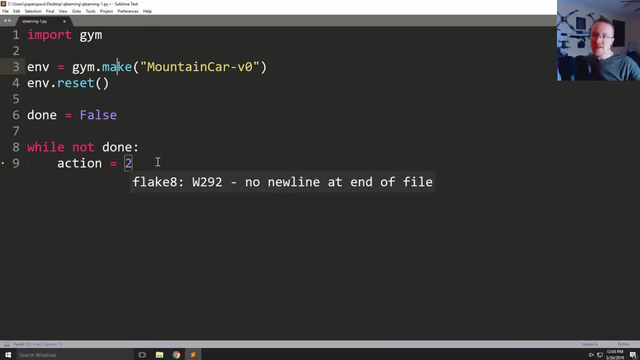 tell you there's three actions. and action zero is like push this car left. action one is do nothing. action two is push the car right. um, so i'm just going to say, basically, push the car right is our action, and we're just going to do that every time. so we're going to say m dot, step, we're going to 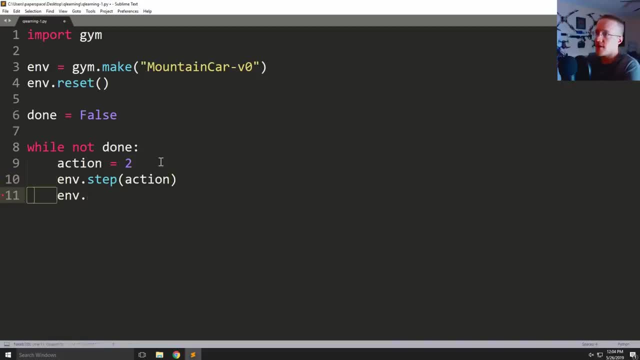 say action and then m dot render, and in fact i think i'll already populate this. uh, that way we don't have to worry. well, we'll hit an error if i don't do this. so the next thing we're going to say is: new underscore, state comma, reward, comma, done comma underscore equals m dot step action. so every 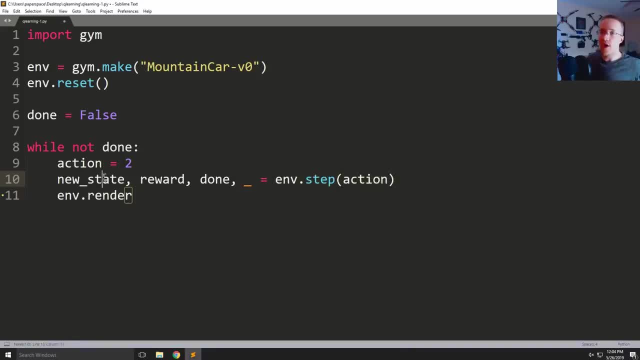 time we step with an action, we get a new state from the environment. so the state is the things that we're like sensing from the environment. basically, in this case, the state is two values: it's position and velocity. but again, like i can, i'm going to continue repeating: uh, your model. it doesn't really matter all that much what these 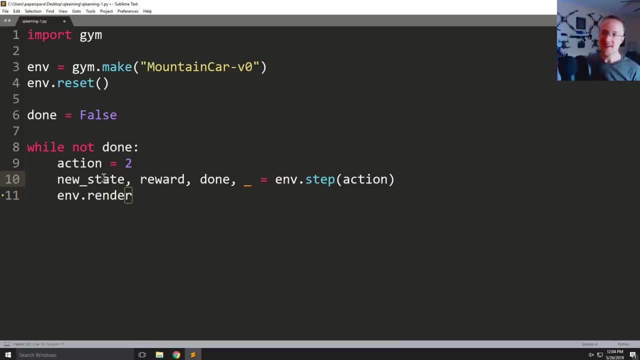 values actually are, as long as they're meaningful. obviously we don't want meaningless data here. but, uh, to the environment or to the agent, it really doesn't matter. but just for your own curiosity's sake. um, the values that we are getting from here are position and velocity of this car. 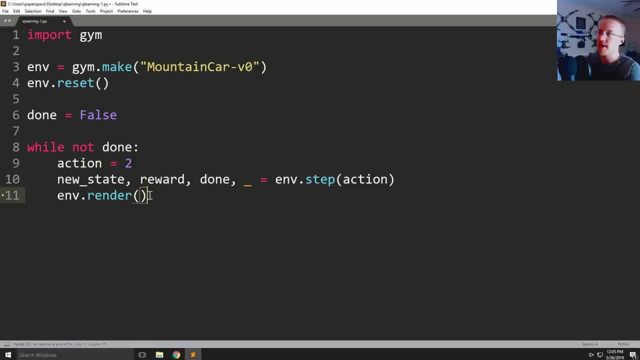 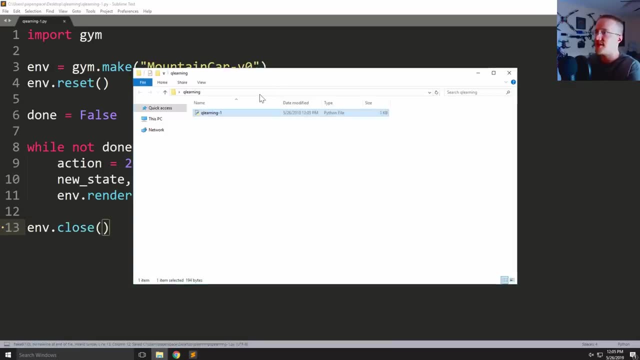 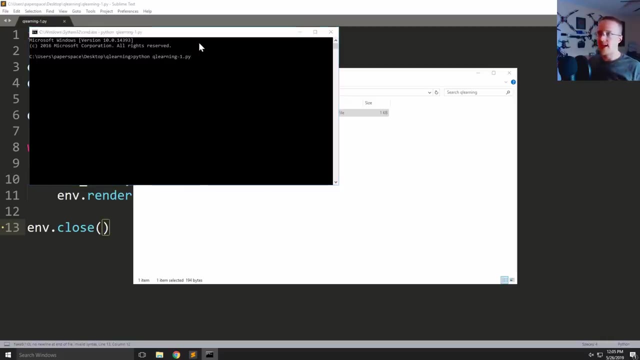 uh, m dot render so that'll show it. and then, if done is done, great. and then, if we are done, we're going to do an env dot close. i'm going to save that, i'm going to run it from a terminal. python q learn one pi and we should get great. so, as you can see, the car is trying to get up this mountain. 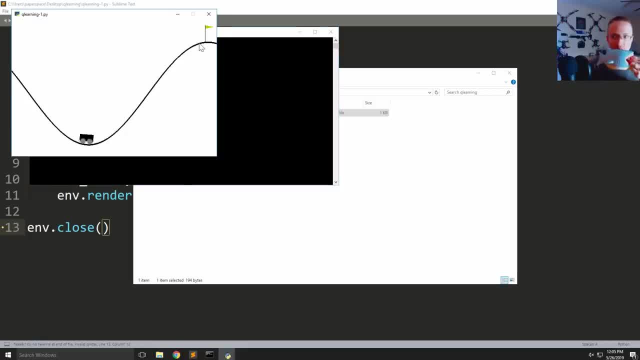 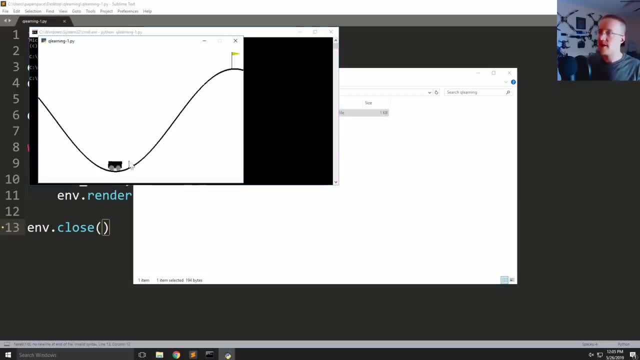 or this hill- i'm not sure i'd call that a mountain, but anyway, it just clearly doesn't quite have the horsepower, and instead what it needs to do is build momentum by going up here, swinging down here and then building up, and, and the goal is to eventually make it uh to this yellow. 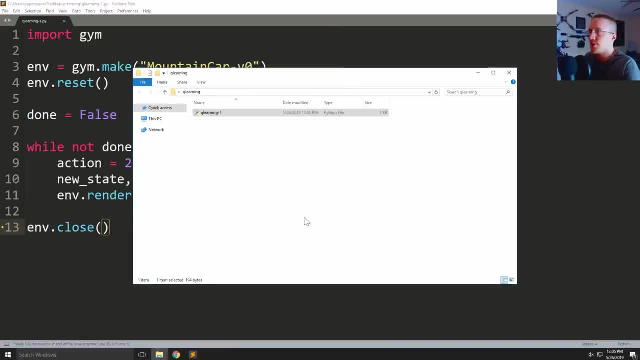 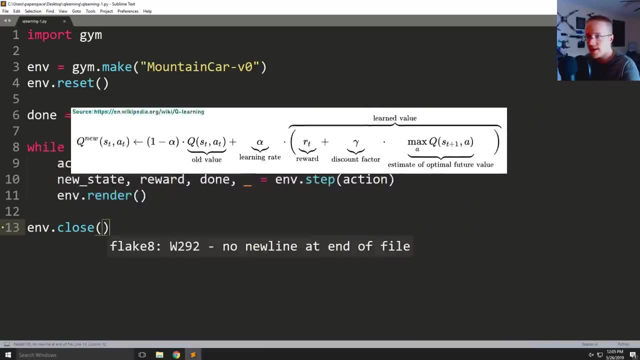 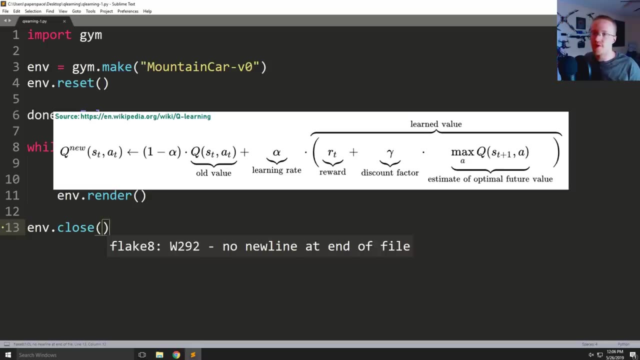 flag area. so okay, so how do we do that? it's actually really, really simple. we just, uh, we just do this. duh, i mean obviously so, um, so this is the actual function here for, uh, calculating these q values. uh, but don't worry, you don't actually need to know how to read that or write from it. 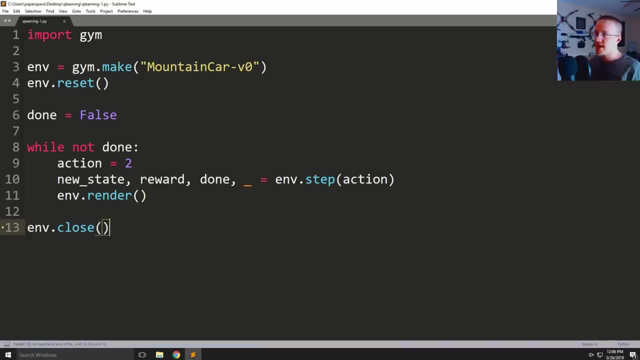 we're going to convert that to python in due time, but basically the way that this is going to work is we want to create this, this q table. it's this large table that, given any combination of states, we can just look it up on the table right. so, given any combination of state, of position and velocity, 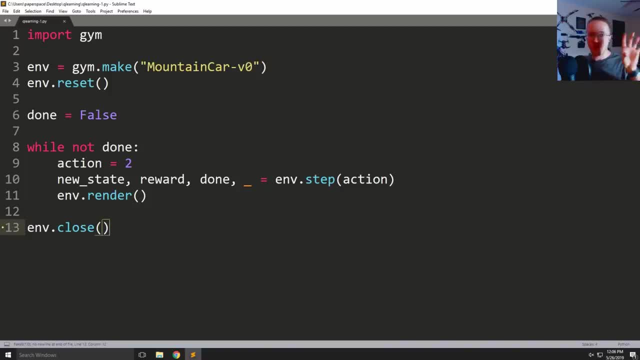 for every combination of position and velocity we were. we just want to look up on this table. hey, what is what? what are the three, in this case q values? at this position in velocity, and as long as we're trying to exploit the environment, we're just going to pick the one with the maximum, the largest q value. that said, when we 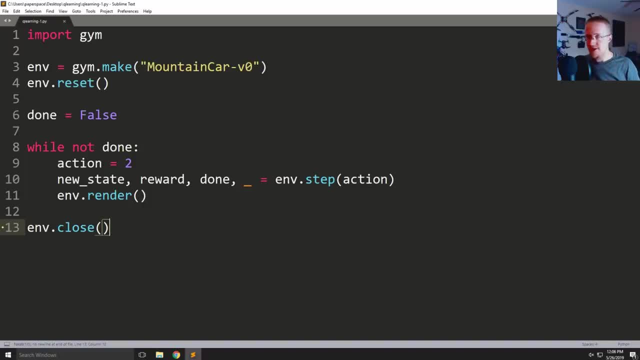 initialize this q table. we just initialize with random values, which also means those values are random and useless. so so actually, initially, our agent is going to do what we call explore a lot, which means do random stuff, uh, and then slowly update those q values as time goes on. 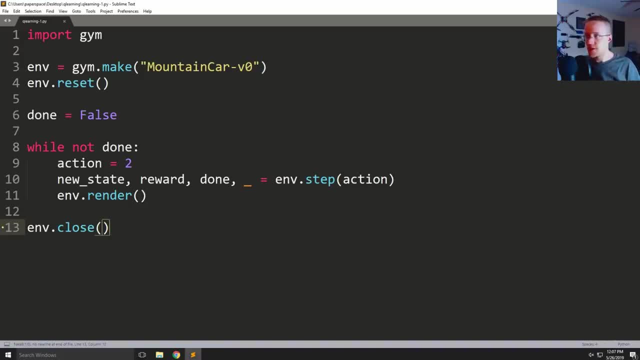 so, anyway, that's a lot of information to throw at you. so so i think the first thing we're going to do is build the q table, um, and then go from there. so so first of all, uh, let me just uh print, we'll print new state save. that did i actually. i think i closed the q table. i think i closed the q table i. 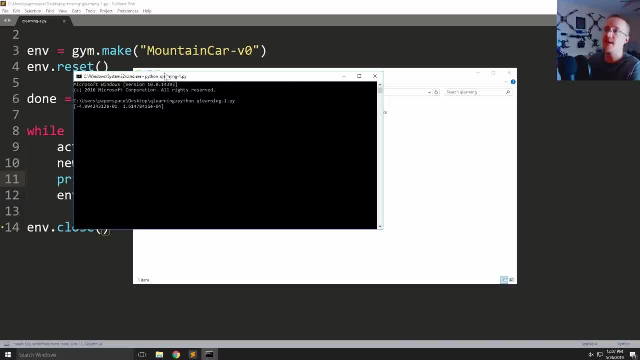 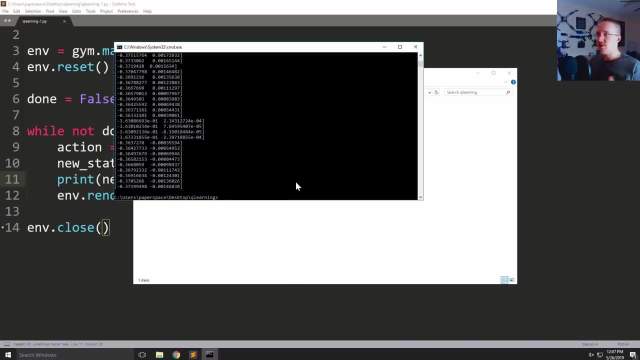 think i closed the console. uh, q learn, i'm just going to run it again and we're just printing out now the states. so, as you can see here we've got all these states being printed out. now this is the first issue that we're going to come across with q learning, and that is that these 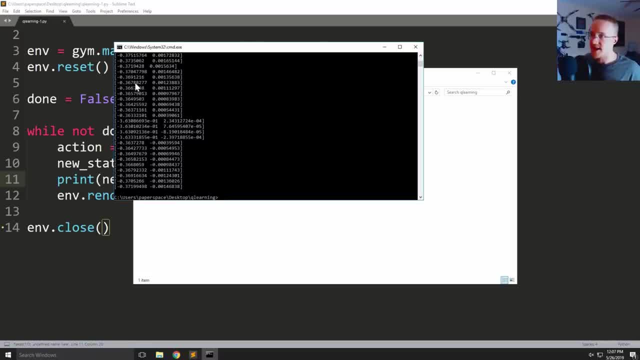 values like that's out to what is that? eight decimal places, that's a lot of decimal places. can you imagine every combination of these two values out to eight decimal places? um, that's a lot. so that would make for a huge table. that's just going to blow out our memory, not only. 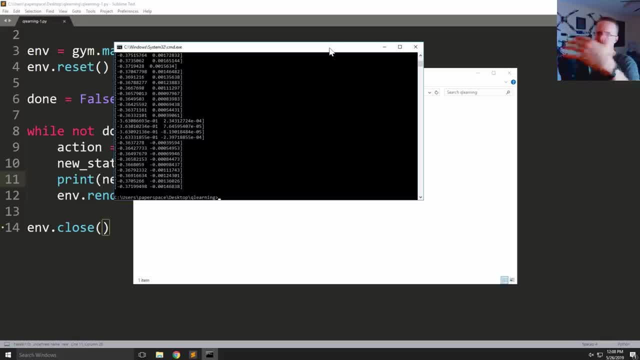 is it going to blow out our memory, but the amount of time it's going to take to learn on a table of that size and the amount of episodes we'd have to like run through to do so- i mean by the time we were done- quantum computing would be like a huge thing already, so so we don't want to wait that. 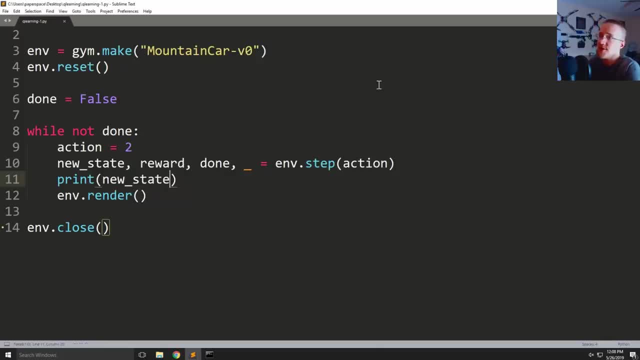 long. so now what we need to do is is convert these continuous values to what are referred to as values. basically, we want to bucket this information into buckets of some sort of size. now, what size those buckets are is, uh, is going to be a yet another one of many variables that we're going 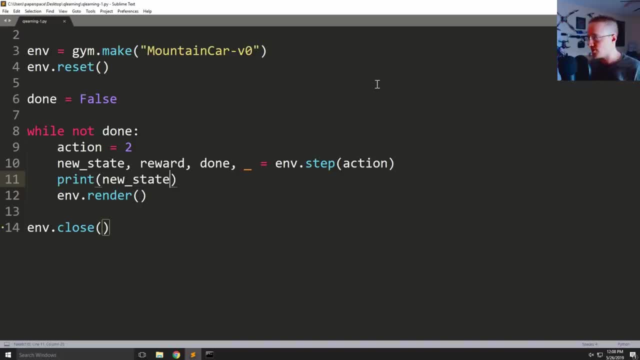 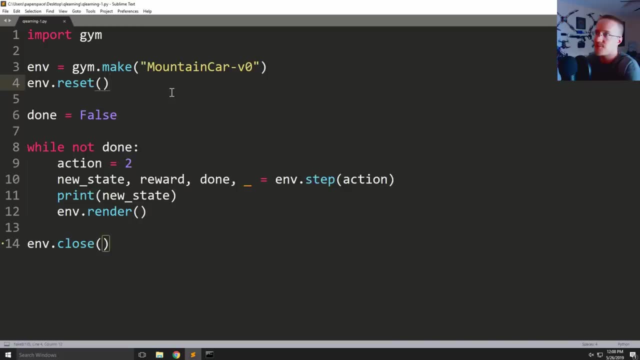 to set and likely need to tweak as time goes on. so, uh, so, with that, let's go ahead and uh, get started here. so, first of all, and so basically, at this point, we can start pulling some information from this environment. one of the things that we can do is print env. 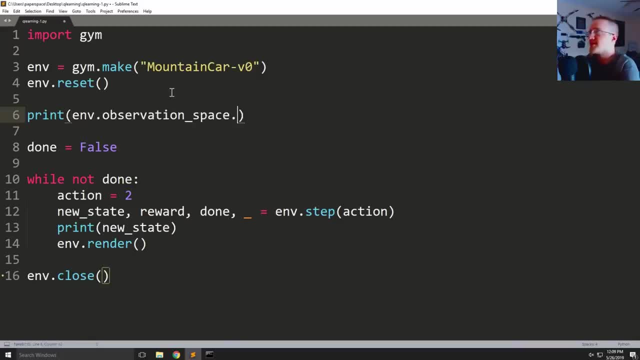 dot observation underscore- space dot high. and then let's just print the low, real quick low. and then one of the other things that we can print is: uh, because i just, i just want to point this out. i think we'll end up using it anyways, but it's uh, yeah, it's action underscore. 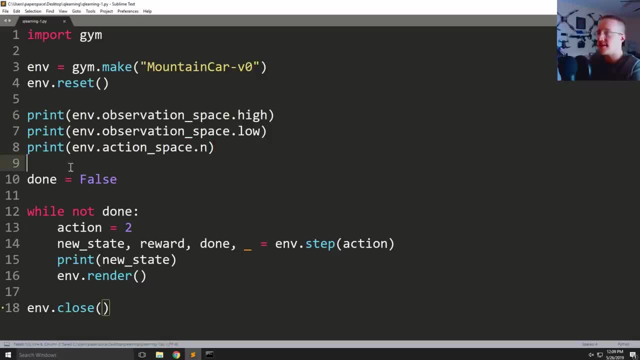 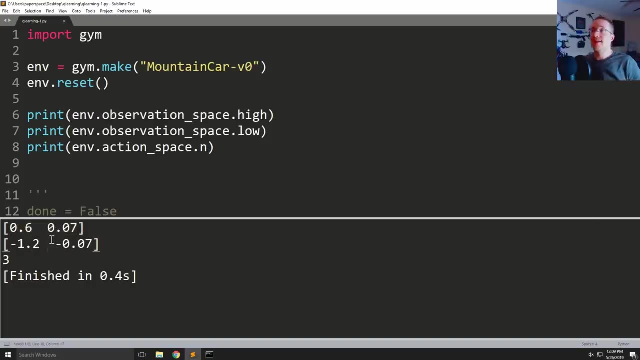 space, dot n, and that'll tell us how many actions we can actually take. so save, we'll just run this in here. so, as you can see, this is the high value for all of the actions or, i'm sorry, all of the observations possible now. another thing to note is you might actually have reinforcement learning. 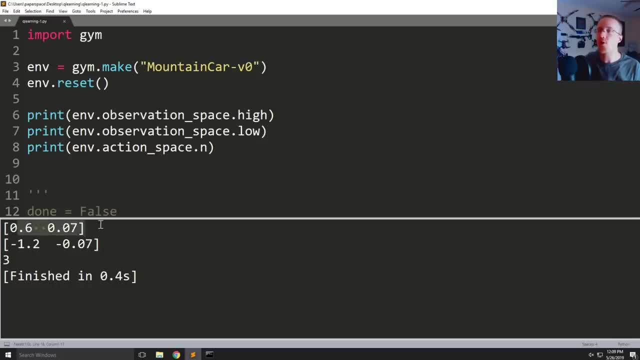 engaging in some sort of environment where you actually don't know these values, and you actually might just engage in this environment randomly for a while before you even start to learn these values. so, um, in this case it the, the environment, is gracious enough to us to report these values, uh, but we might actually not know. and then here with actions, chances are. 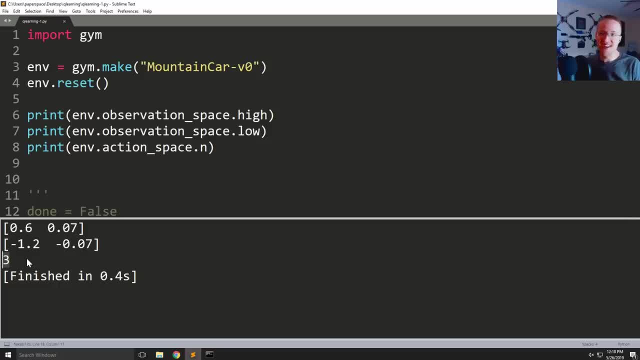 you'll know your actions in advance. no matter, no matter what um. i can think of a few use cases for, like reinforcement learning, at least where you wouldn't, but probably not q learning, but anyway, we can pull the environment of any of these gym environments this way to know exactly how many actions are possible. okay, so the next thing that we want to do: 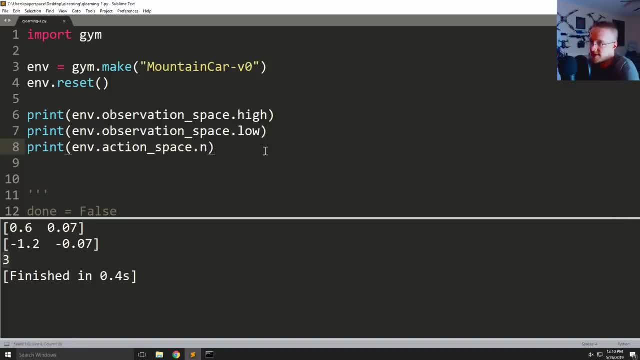 is create. we want to figure out how we're going to create this q table. so, um, so we want this q table to be of a size that's at least manageable. so how we're going to make that size, i'm just going to say um, discrete observation, observation space or os size, and in this case we we're going to say: 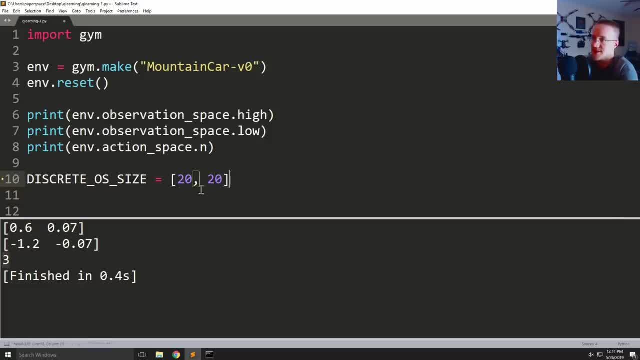 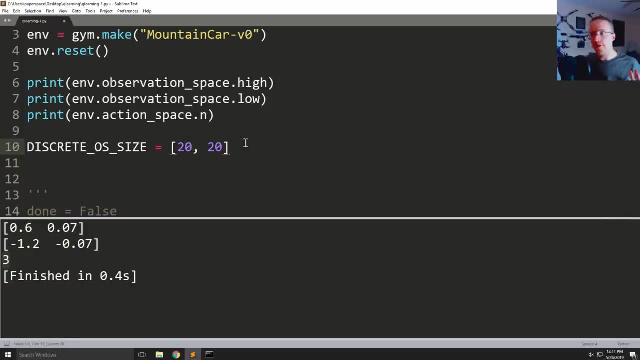 2020.. now, um, i'm going to change this in just a second. i am kind of on the fence as far as like hard coding this. i think that a real or reinforcement learning agent would not have this hard coded because it would change by environment, um, but 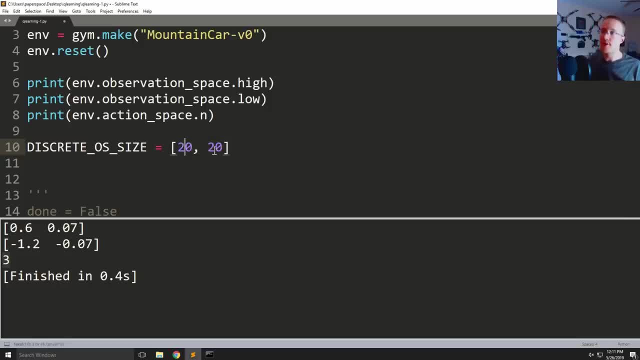 you won't necessarily always want these values to be the same number, like this one. maybe you want 50, and then this one should be 20 and so on, but for now, what i'm going to say is just going to be 20, um times the len of. 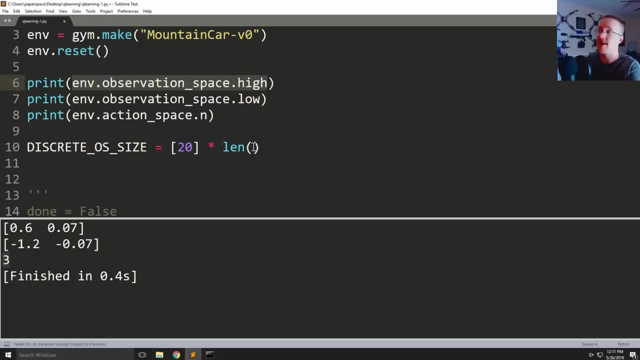 any observation space thing, so i'm just going to pick one at random. so this is two, so it's just 20 times two, so it's a 20 by 20.. okay, um, i'm only doing that just because i really want this code to be at least functional on every environment possible. um, so i just don't want to hard code. 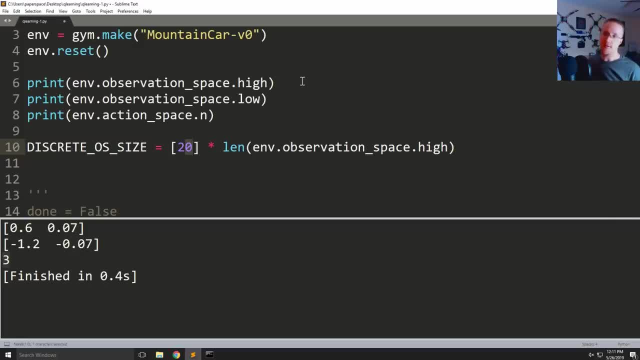 that because some environments won't only have two observation values. they might have five, ten, a hundred. hopefully not, but maybe so. anyway, cool, so all right. so we've got the discrete values. okay, so we're going to take the numbers from the range of 0.07 to negative 0.07, and then 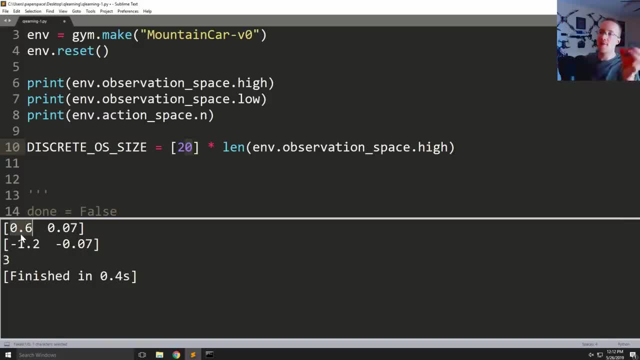 we want to separate that range into the observation, uh, space size. so with that entire range, so from 0.6 to negative 1.2, we want to separate that range into 20 chunks, or 20 buckets, or 20 discrete values. okay, however you want to call it, that's what we want to do. and then we want to do the same thing. 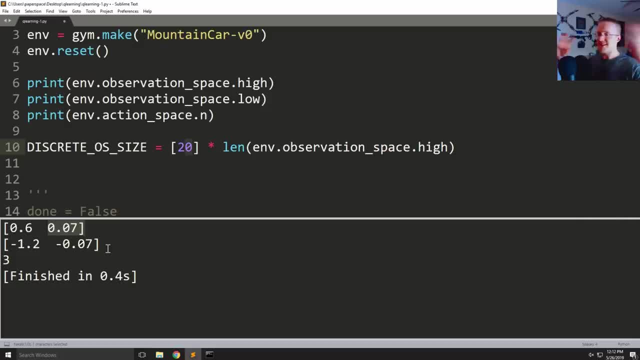 chunks and buckets. that way we don't just have this infinitely continuous range. that would be forever for us to learn. so now we need to know how big is that range, how big are those chunks? you know like each step through those chunks. so how big is that number? so now we're going to say 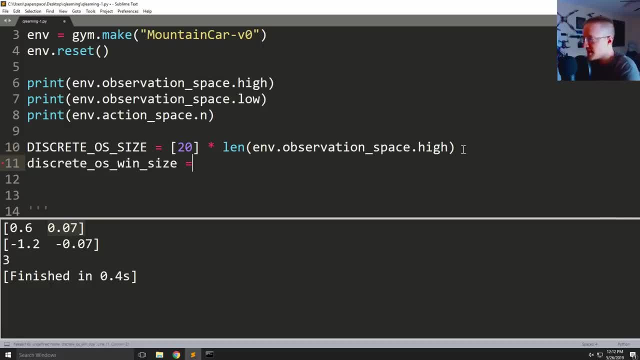 discrete os win size is equal to n? um. really are you not gonna help me? observation space dot high. i was really hoping it would just like auto complete that entire thing for me anyway. uh, minus m dot. observation space dot low, and then i'll add the spaces around that. 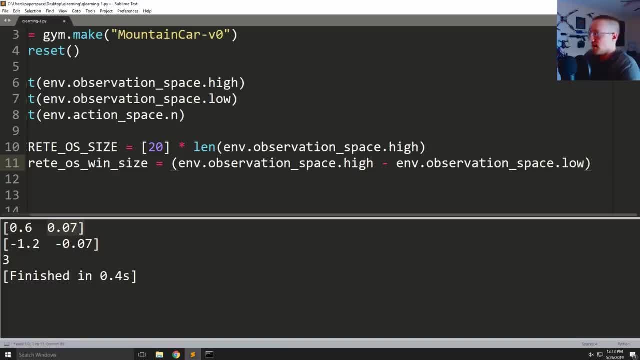 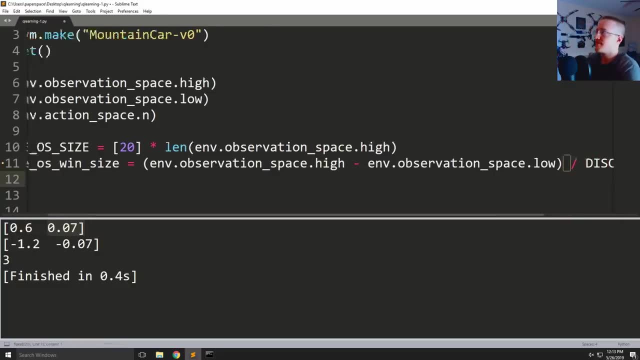 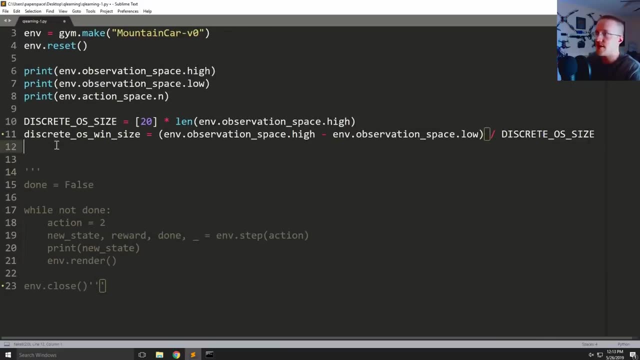 i'm pretty sure that would be pep8. then what we want to say is: divided by discrete os size, that's freaking huge, um. and then what i'm gonna do is i'm just gonna print this out, just so you can see what i'm talking about. so now print. not in all caps, though, uh print. 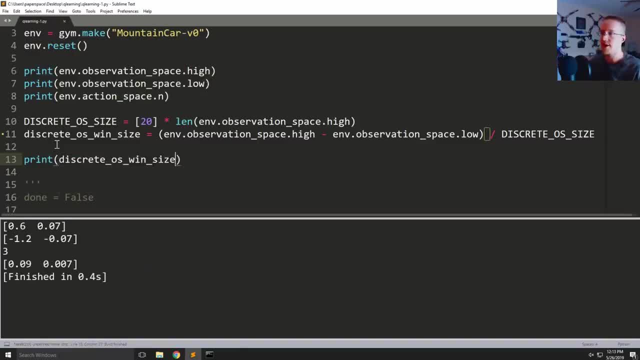 discrete os win size. we'll run that real quickly and you can see now you okay. so. so for positions, each bucket will be of a range that is 0.09 long and then over here 0.007 long for the velocity chunks, and knowing that i would say i'm just going to guess that's. 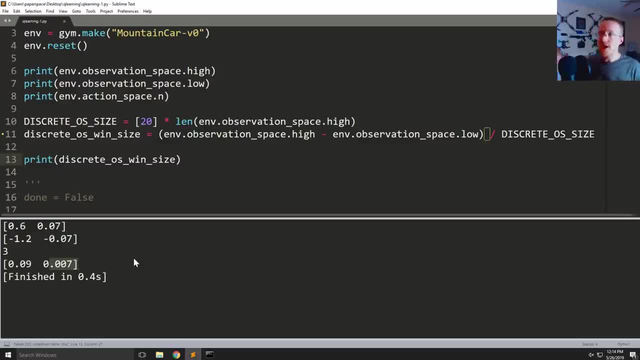 probably granular enough and in fact i'm not guessing. i already know it's going to work, so so it will be. but sometimes you might find that you have to tweak these values and again, like i said, sometimes they won't necessarily be the same between two. so i just i made this. 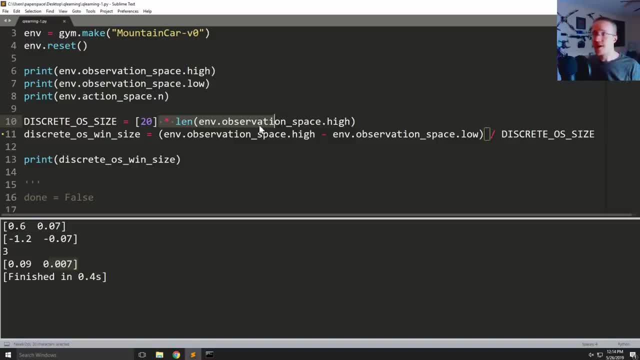 change because i want it to work across all environments, and by work i mean just the code, but really you would take your q learning scripts and make them far more, uh, dynamic and probably also run like a few, maybe even a few hundred episodes, to tweak these numbers a bit. 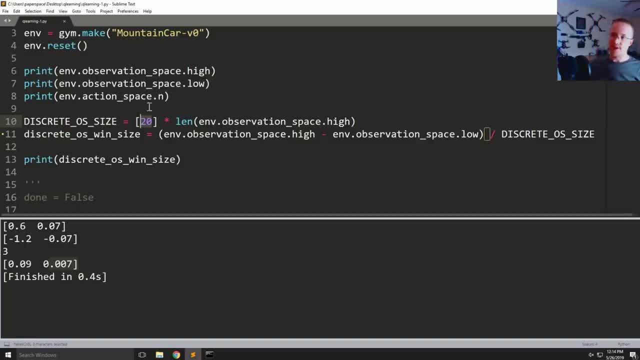 but because this is not our stopping point, i'm not going to spend a bunch of time doing that, like we're going to get into deep q learning and stuff, so i don't, i don't want to spend too much time there. uh, we will spend a little bit of time talking about how we can optimize these numbers. 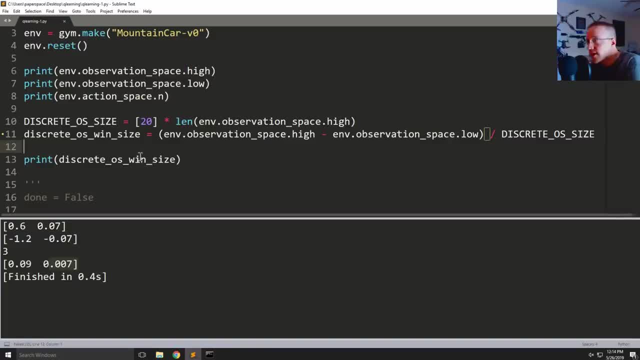 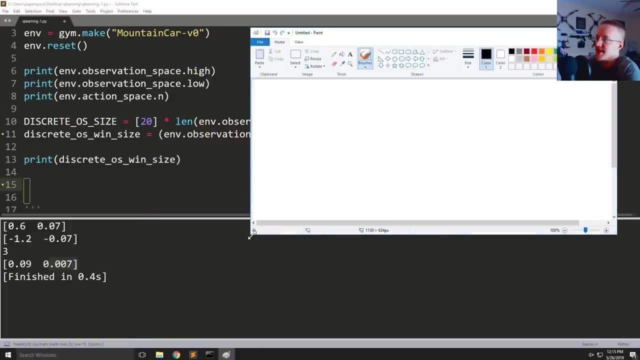 but yeah, anyways, moving on. so discrete win size is now known. so finally, we can create the cue table. so again, i'm going to open up paint, because paint is love and paint is life. um, the the objective at the end of the day for us is to have this like massive cue table. okay, and so? 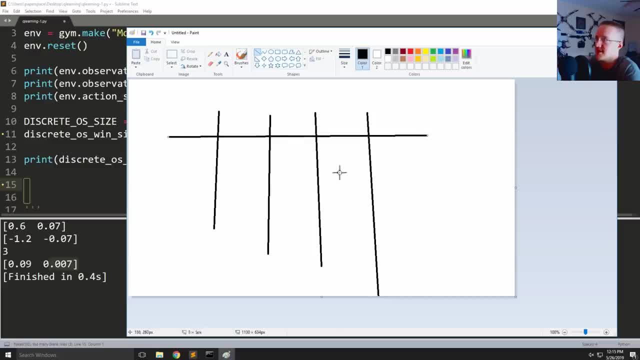 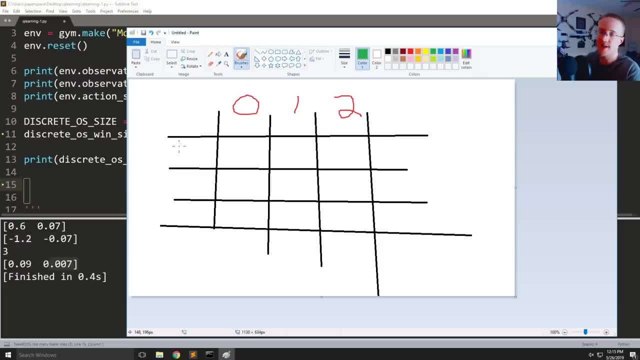 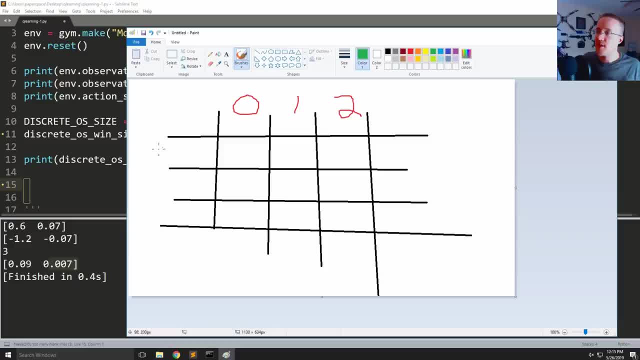 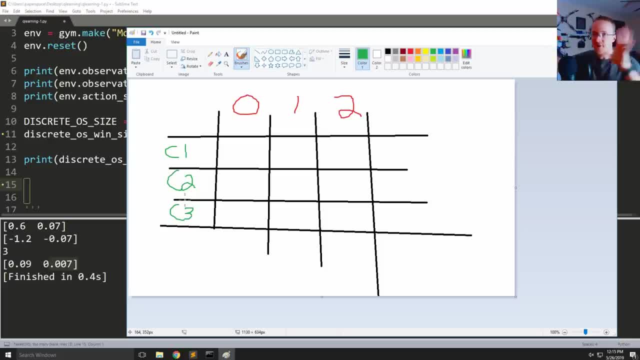 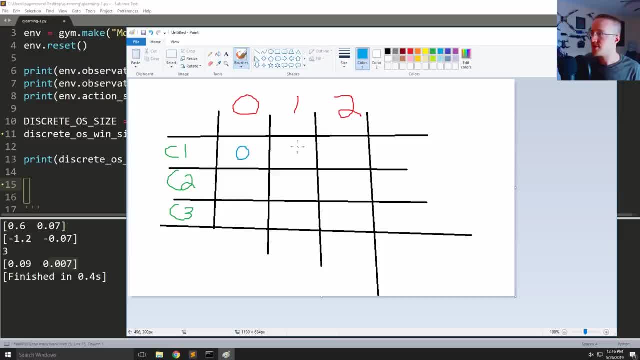 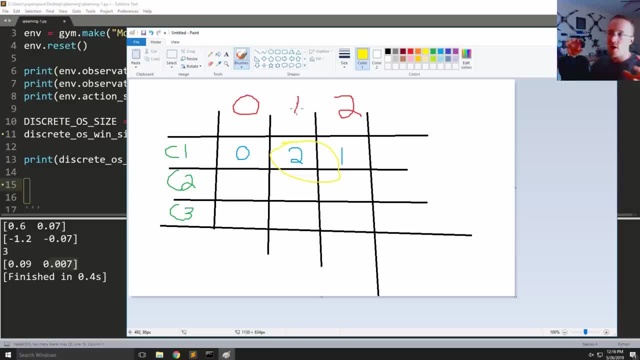 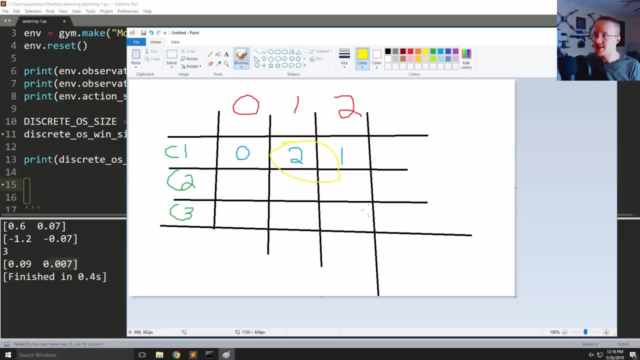 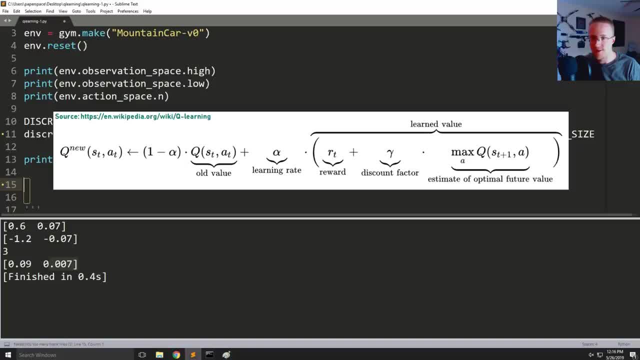 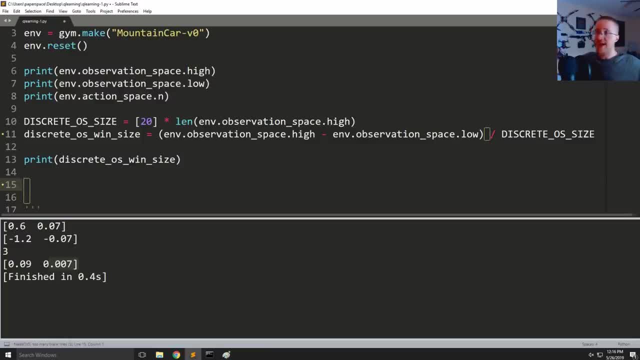 uh, it will slowly kind of back propagate that reward to make for higher q values, that reward to make for higher q values, that reward to make for higher q values for the actions that when chained, for the actions that when chained for the actions that when chained together. 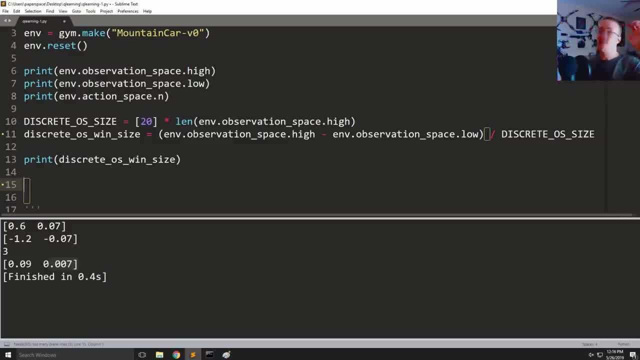 together, together, lead to that lovely reward, but for now we lead to that lovely reward. but for now we lead to that lovely reward, but for now we need to need to need to. we just need to initialize this q table. so we just need to initialize this q table. so 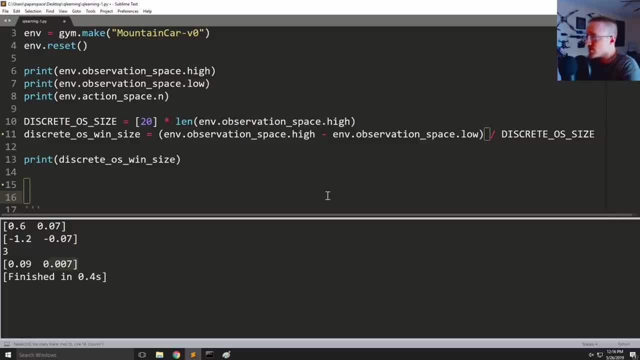 we just need to initialize this q table so later we can update this q table, later we can update this q table. so the way that we're going to initialize, the way that we're going to initialize, the way that we're going to initialize this q table, is we're going to say q. 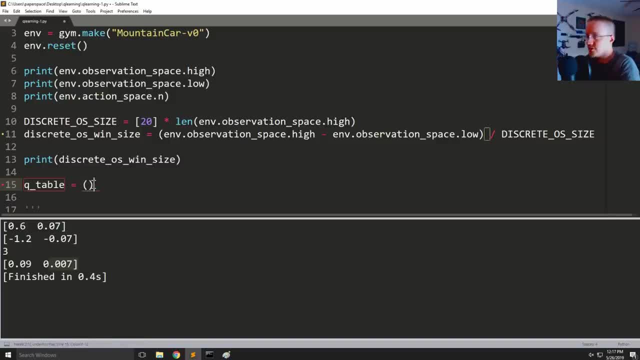 this q table is we're going to say q, this q table is we're going to say q, underscore, underscore, underscore. table is equal to table, is equal to table is equal to um, oops, um, oops, um, oops. np, dot, random, dot, uniform. np, dot, random, dot, uniform. 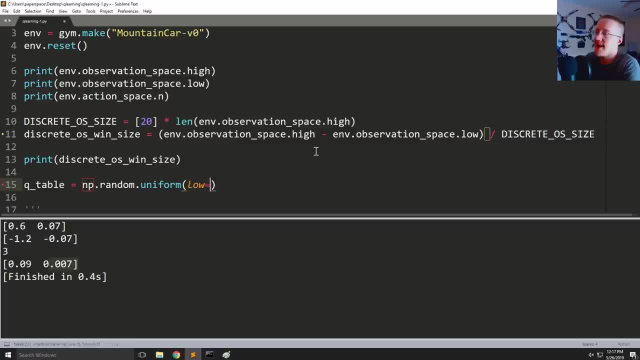 np, dot, random, dot, uniform, and then we're going to say low equals, and then we're going to say low equals, and then we're going to say low equals, and we're going to start at negative, and we're going to start at negative, and we're going to start at negative. two high equals zero, and again these. 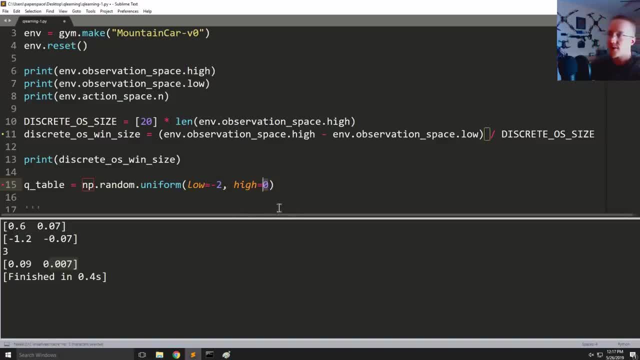 two high equals zero, and again these two high equals zero, and again these are two variables that you're going to, are two variables that you're going to, are two variables that you're going to want to probably tinker with, want to probably tinker with, want to probably tinker with, given different environments, and 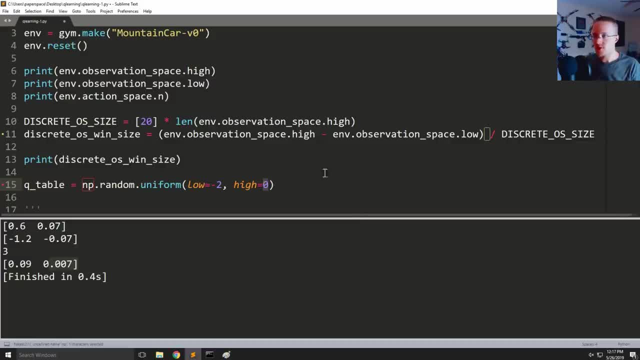 given different environments and given different environments and um, and that's why, in one of the um, and that's why in one of the um, and that's why in one of the subsequent tutorials we will have to subsequent tutorials, we will have to subsequent tutorials, we will have to talk about, like: how do you analyze these? talk about like: how do you analyze these? talk about like: how do you analyze these environments? because it's not, you know environments. because it's not. you know environments because it's not, you know, there's no tensor board to pull up, and there's no tensor board to pull up, and 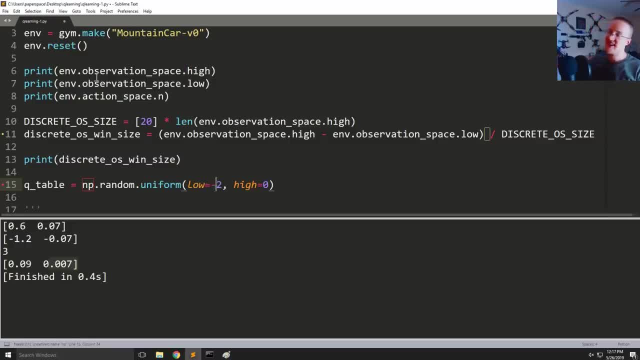 there's no tensor board to pull up and check, the, check, the check, the, the loss, you know so anyway. um, these, the loss, you know so anyway. um, these, the loss, you know so anyway. um, these, the, the, the intuition behind why these, the, the, the intuition behind why these. 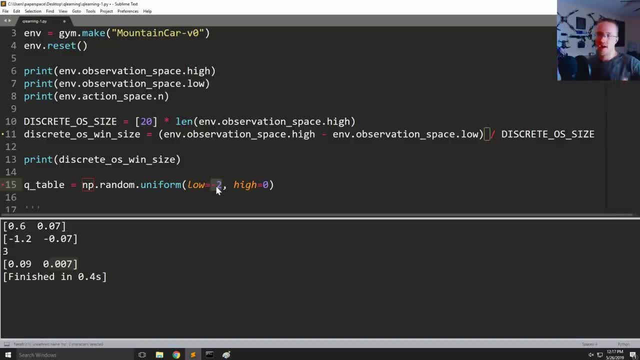 the, the. the intuition behind why these should work is the rewards that we're the. the intuition behind why these should work is the rewards that we're going to be getting um, going to be getting um, going to be getting um. basically, when we print, we even printed. 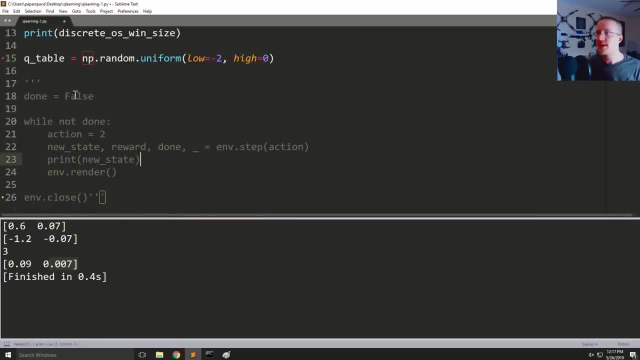 basically, when we print, we even printed. basically, when we print, we even printed it out. uh, here, um, oh no, we only printed it out. uh, here, um, oh no, we only printed it out. uh, here, um, oh no, we only printed out the new state um out the new state um. 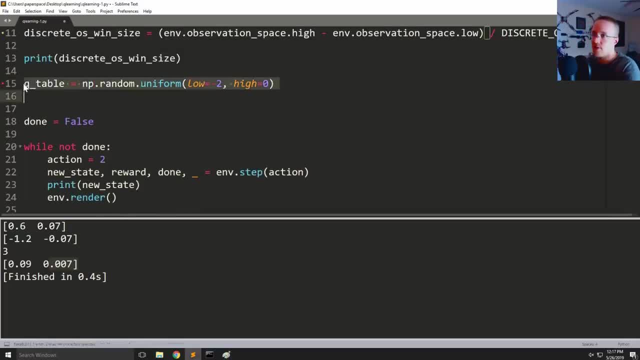 out the new state. um, since it's, since it's part of what i'm, since it's, since it's part of what i'm, since it's, since it's part of what i'm trying to yak about right now, trying to yak about right now, trying to yak about right now, let's just i'm going to comment that out. 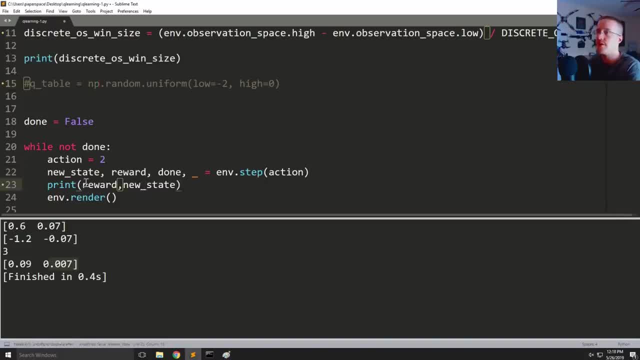 let's just, i'm going to comment that out. let's just, i'm going to comment that out and i'm going to print, and i'm going to print, and i'm going to print: reward and then new state. so now you can reward and then new state. so now you can. 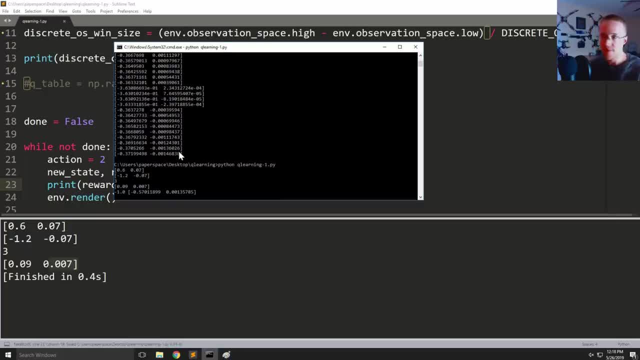 reward and then new state. so now you can see all of the rewards and i'll do that. see all of the rewards, and i'll do that see all of the rewards, and i'll do that in the console. so coming over here we can see that the 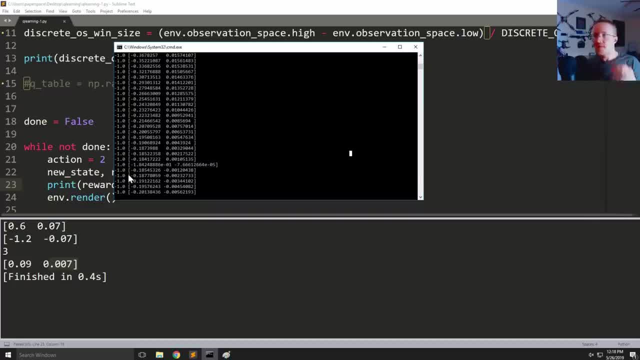 so, coming over here, we can see that the so coming over here, we can see that the reward here is always a negative one. reward here is always a negative one. reward here is always a negative one. and again um to your agent, it doesn't. and again um to your agent, it doesn't. 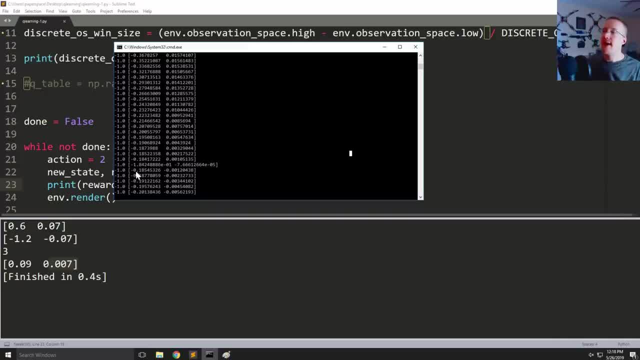 and again: um, to your agent, it doesn't really matter, really matter, really matter all that much, but to you it might and all that much, but to you it might and all that much, but to you it might, and that. so basically it's good the reward, that so basically it's good, the reward. 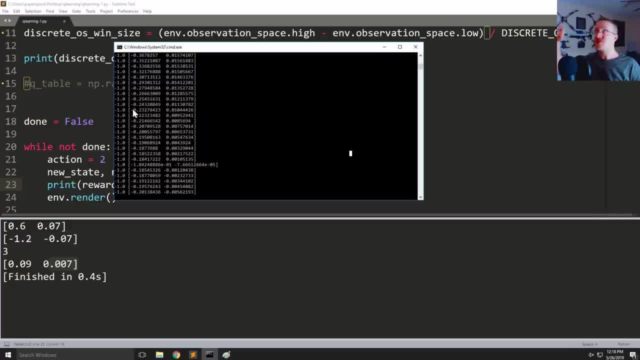 that. so, basically, it's good. the reward is going to be a negative one is going to be a negative one is going to be a negative one until you re you reach that flag, until you re you reach that flag, until you re you reach that flag, at which point your reward will be zero. 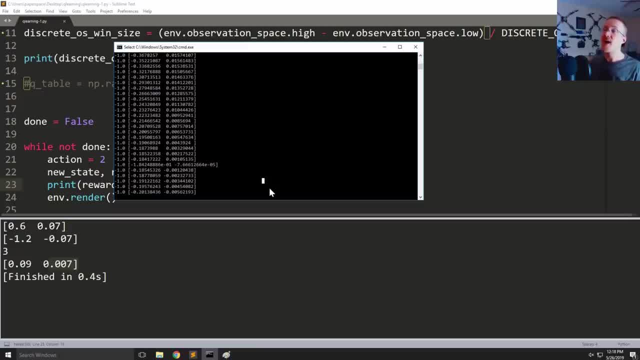 at which point your reward will be zero, at which point your reward will be zero, um, um, um, so, so, yeah, so, so that's how, so, so, yeah, so, so, that's how, so, so, yeah, so, so that's how, um. once it finally reaches that flag, it. 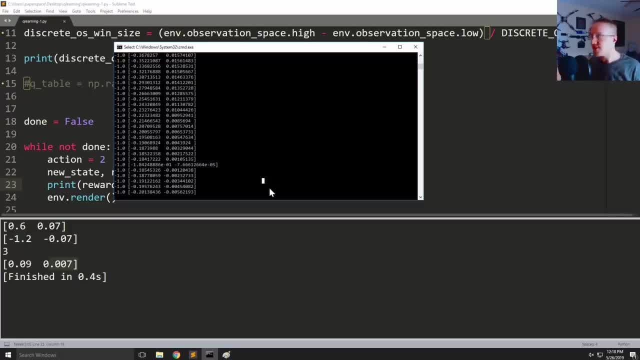 um, once it finally reaches that flag, it um, once it finally reaches that flag, it gets a zero reward, which is gets a zero reward, which is gets a zero reward which is higher than negative one, i guess i think higher than negative one, i guess i think higher than negative one. i guess i think we should get a bigger, better reward. 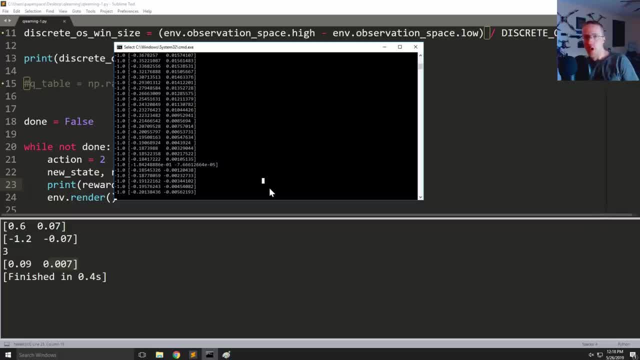 we should get a bigger, better reward. we should get a bigger, better reward, personally, uh, but once it reaches that, personally, uh, but once it reaches that, personally, uh, but once it reaches that flag, and then we back propagate those flag and then we back propagate those flag and then we back propagate those. that chain of events, basically so. 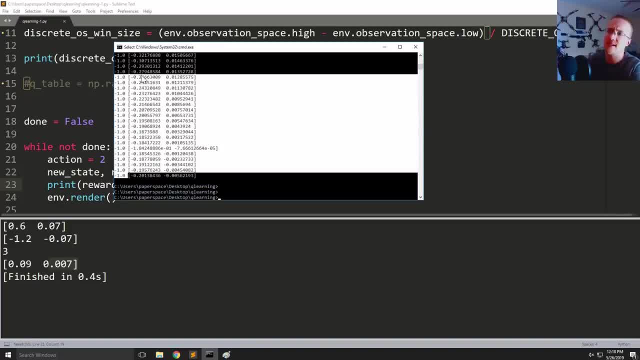 that chain of events, basically so, that chain of events, basically so, anyways, um. we can see here that the anyways, um. we can see here that the anyways, um. we can see here that the rewards are always negative one until a rewards are always negative one until a rewards are always negative one until a good thing happens. so we, we can. 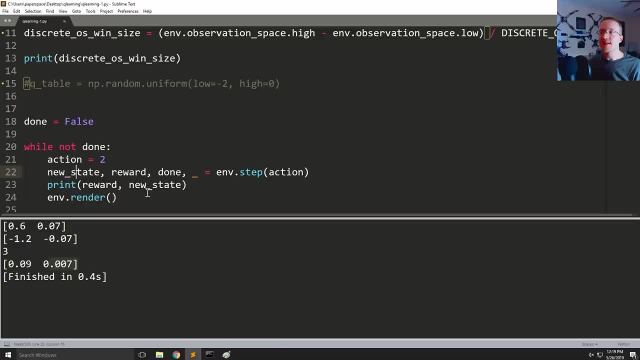 good thing happens, so we we can. good thing happens, so we we can initialize the table into the negatives, initialize the table into the negatives, initialize the table into the negatives because we're pretty confident that, because we're pretty confident that, because we're pretty confident that that's where, like, the values will. 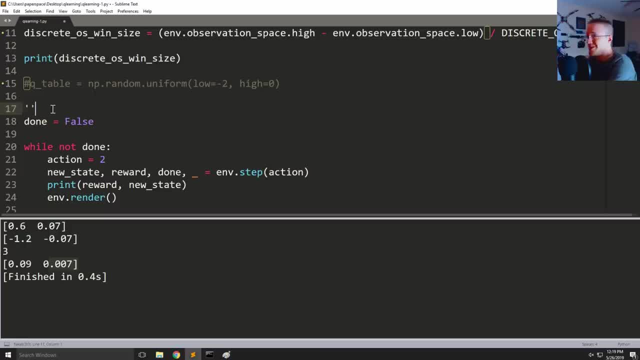 that's where like the values will. that's where like the values will lead to start it there, uh, but again you lead to start it there, uh, but again you lead to start it there, uh, but again you. you'd want to be, you'd probably want to. 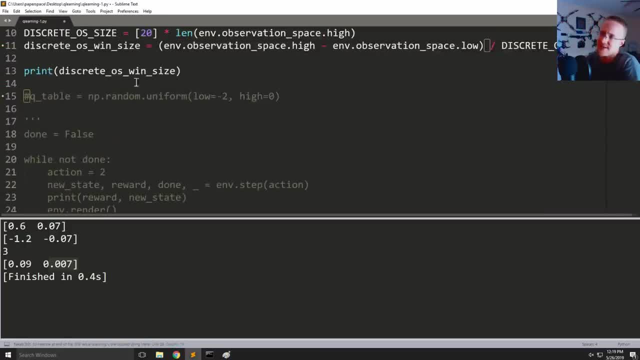 you'd want to be. you'd probably want to. you'd want to be, you'd probably want to tinker with a lot of starting values. to tinker with a lot of starting values. to tinker with a lot of starting values. to be honest, and then, given enough time, it. 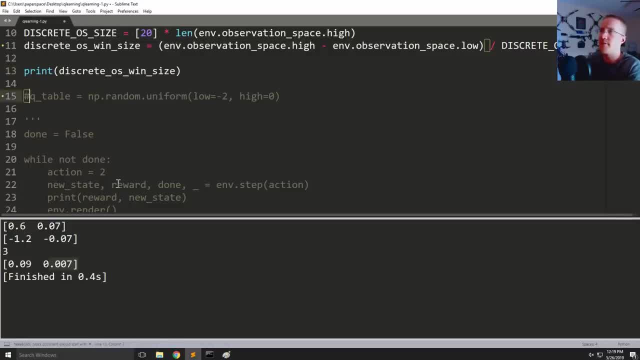 be honest and then, given enough time, it be honest, and then, given enough time, it should figure it out anyways. but anyway should figure it out anyways, but anyway should figure it out anyways, but anyway, um coming back to our q table, um, coming back to our q table. 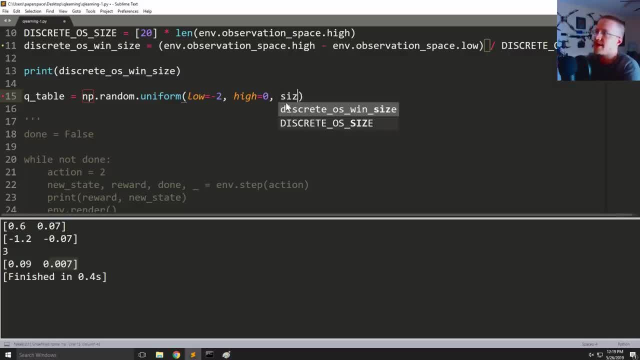 um, coming back to our q table, so our low is going to be negative 2, our. so our low is going to be negative 2, our, so our low is going to be negative 2. our high is going to be 0 and then high is going to be 0 and then 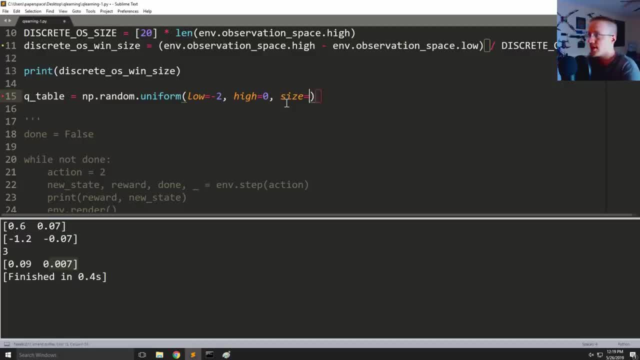 high is going to be 0, and then, finally, our size is going to be equal. finally, our size is going to be equal. finally, our size is going to be equal to, to, to, um, the discrete os size, um, the discrete os size, um, the discrete os size, which, if we come over here, that's a 20. which, if we come over here, that's a 20, which, if we come over here, that's a 20 by 20.. so the table is 20 by 20.. so by 20.. so the table is 20 by 20.. so. 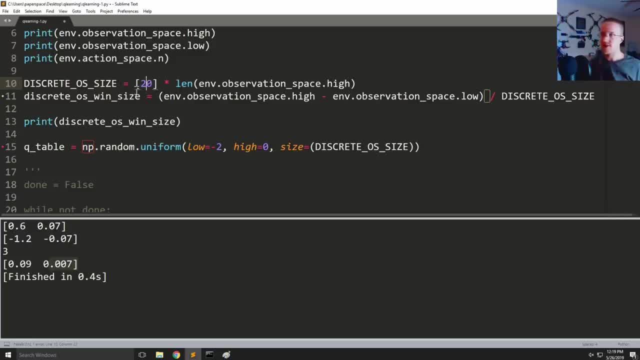 by 20.. so, when we do make a 20 by 20 table, of when we do make a 20 by 20 table, of when we do make a 20 by 20 table of this discrete observation space size, this discrete observation space size, 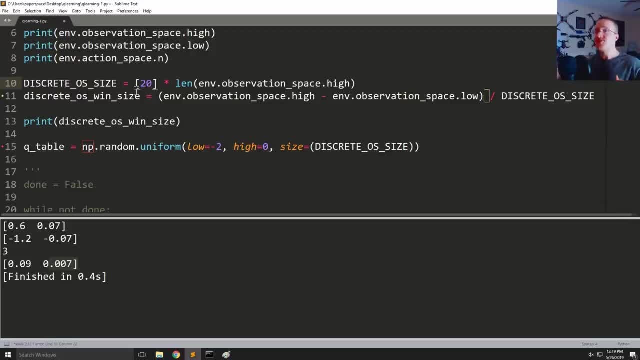 this discrete observation space size that contains every combination, that contains every combination of uh um observations that we might of uh, um observations that we might of uh, um observations that we might find. so every combination of uh find, so every combination of uh find, so every combination of uh position and velocity. 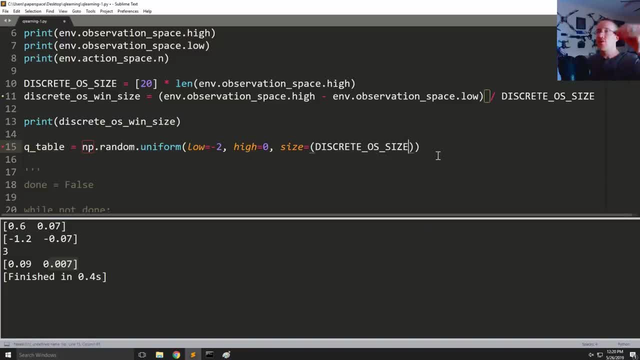 position and velocity. position and velocity, then then then we need values for every single action. we need values for every single action. we need values for every single action. that's possible, that's possible, that's possible. so the way that we're going to do that, so the way that we're going to do that, 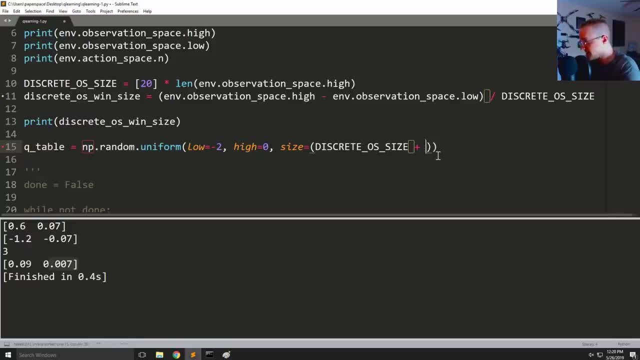 so the way that we're going to do that is discrete observation space size is discrete observation. space size is discrete observation space size plus um, plus um, plus um env dot, whoops, env, env dot, whoops, env dot, env dot, env, dot. action space dot n. action space dot n. 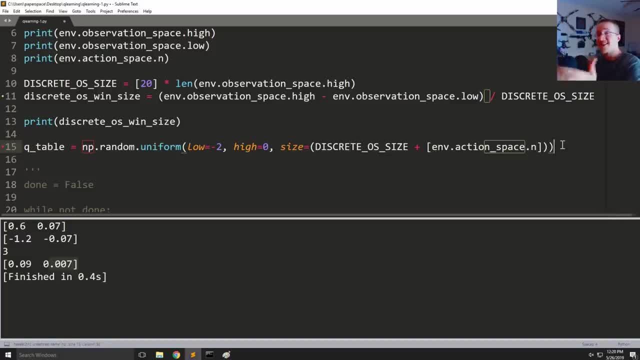 action space dot n, so so. so this should make us a 20 by 20, this should make us a 20 by 20, this should make us a 20 by 20 by 3, so it's a three-dimensional table by 3, so it's a three-dimensional table. 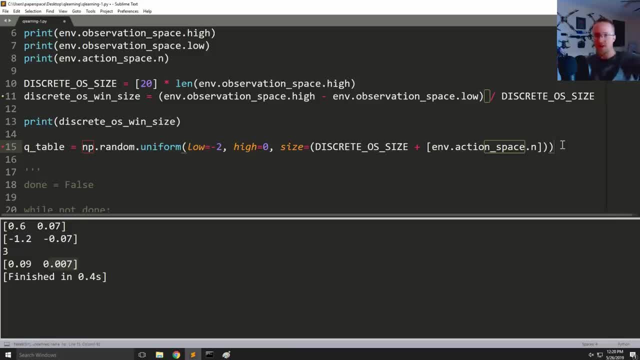 by 3, so it's a three-dimensional table, but basically you can just think of it. but basically you can just think of it, but basically you can just think of it as it's every combination of possible, as it's every combination of possible, as it's every combination of possible. environment observations- times three. 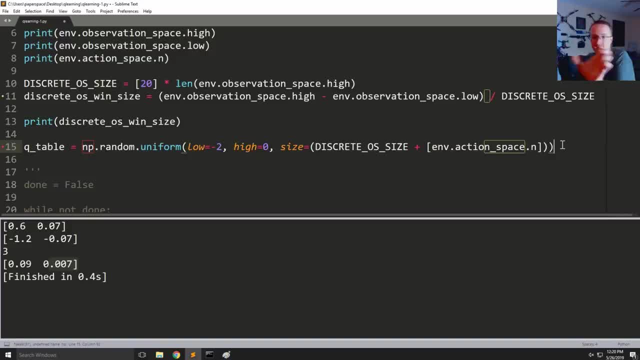 environment observations times three. environment observations times three: uh, actions that we could take, and then uh, actions that we could take, and then uh, actions that we could take, and then inside of those cells, or whatever you inside of those cells, or whatever you inside of those cells, or whatever you want to call them. 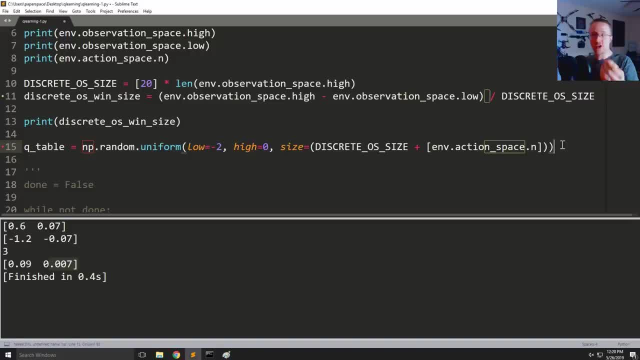 want to call them. want to call them. you're going to have your three at this. you're going to have your three at this. you're going to have your three at this point. random q values between negative point. random q values between negative point. random q values between negative two and zero. 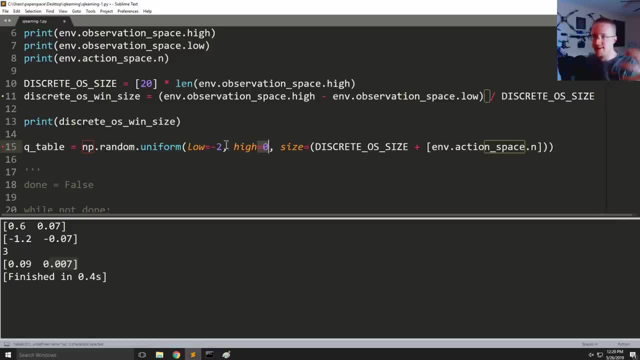 two and zero. two and zero, but over time through this agent's, but over time through this agent's, but over time through this agent's. exploration and exploitation, exploration and exploitation, exploration and exploitation. those values should get slowly tweaked. those values should get slowly tweaked. those values should get slowly tweaked and optimized. 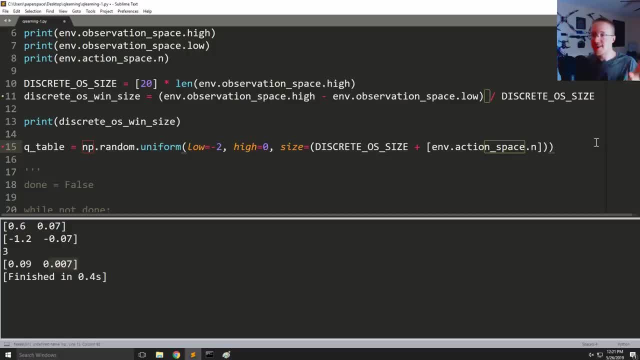 and optimized, and optimized based on that, based on that, based on that. but don't worry, we'll write that in. but don't worry, we'll write that in. but don't worry, we'll write that in python, and it makes so much more sense, python, and it makes so much more sense. 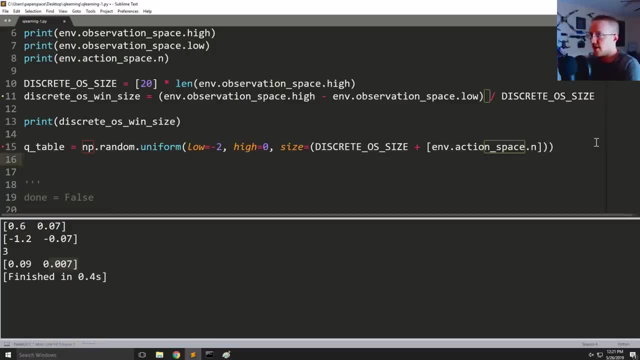 python, and it makes so much more sense, at least to me- in python than it does in, at least to me in python, than it does in, at least to me in python, than it does in that stupid formula, that stupid formula, that stupid formula. but for now let me go ahead and just. 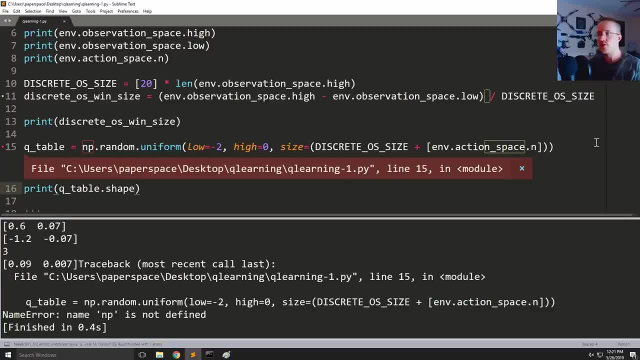 but for now, let me go ahead and just but for now, let me go ahead and just print uh q table dot shape. and let's print uh q table dot shape. and let's print uh q table dot shape and let's make sure, make sure, make sure it's what we expected. np is not defined. 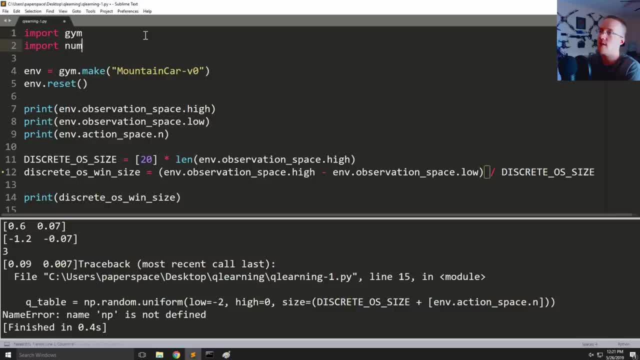 it's what we expected. np is not defined. it's what we expected: np is not defined. let's go ahead and import. let's go ahead and import. let's go ahead and import. uh, import numpy as np, we'll try one more. uh, import numpy as np, we'll try one more. 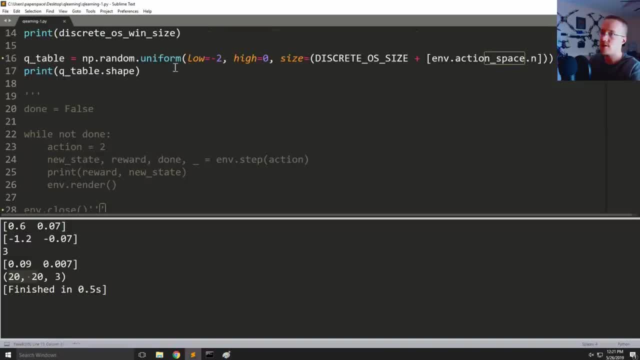 uh, import numpy as np. we'll try one more time time time: 20 by 20 by 3, and then, if you wanted to 20 by 20 by 3, and then if you wanted to 20 by 20 by 3, and then if you wanted to look at it, you could. but look at it you could, but look at it you could, but we're not really going to gleam anything. we're not really going to gleam anything. we're not really going to gleam anything from it. it's not going to look very from it it's not going to look very. 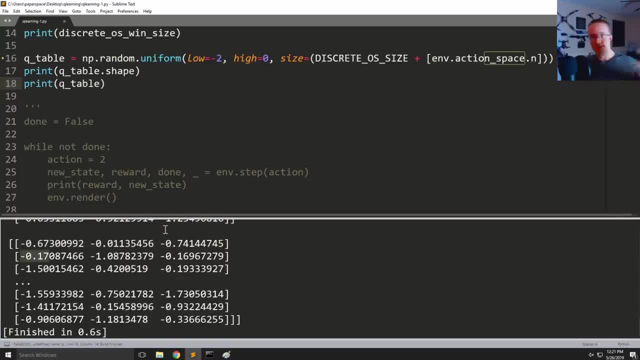 from it it's not going to look very meaningful to us just understand. meaningful to us, just understand. meaningful to us just understand. um, it's every you know possible. um, it's every you know possible. um, it's every you know possible. observation combination, observation combination, observation combination and then the q values for at every 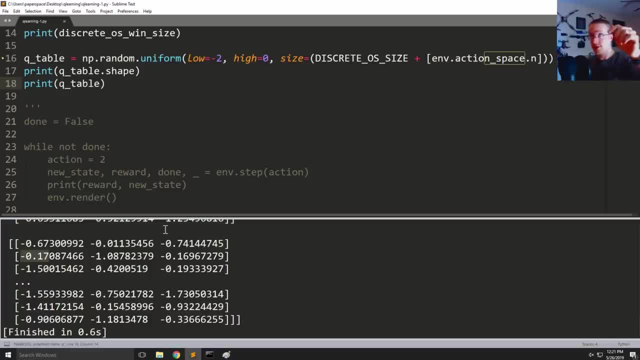 and then the q values for at every, and then the q values for at every possible observation combination and possible observation combination and possible observation combination and every combination of every combination, of every combination of, or every possible action at every or every possible action, at every or every possible action, at every possible combination. we have a random. 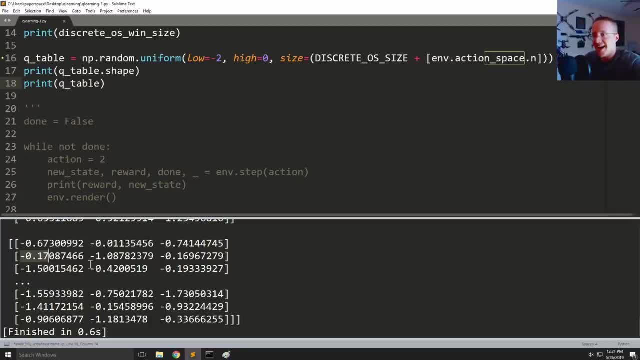 possible combination. we have a random possible combination. we have a random starting q value, starting q value, starting q value. okay, so, um, i think i'm going to cut it. okay, so, um, i think i'm going to cut it. okay, so, um, i think i'm going to cut it here and in the next video we will talk. 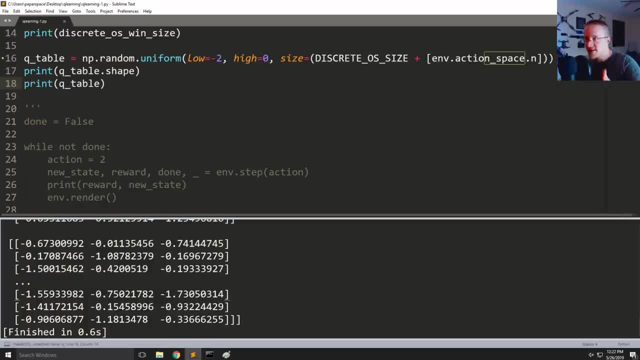 here and in the next video we will talk here and in the next video we will talk about how to actually start training, about how to actually start training, about how to actually start training- this model iterating and going over this model iterating and going over this model iterating and going over these- uh, the steps per episode and all. 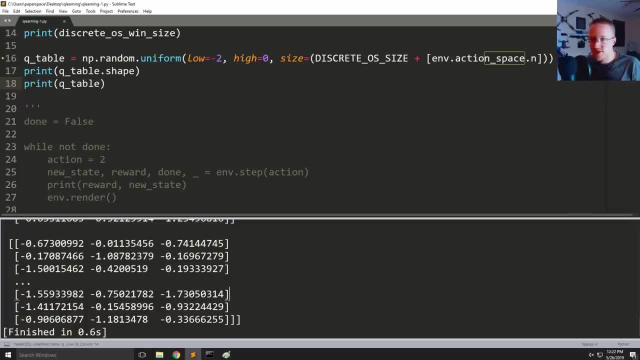 these, uh, the steps per episode, and all these, uh, the steps per episode, and all the episodes and all that, the episodes, and all that, the episodes, and all that. so, uh with that a shout out to so uh with that a shout out to so uh with that, a shout out to my longest term channel members. these are: 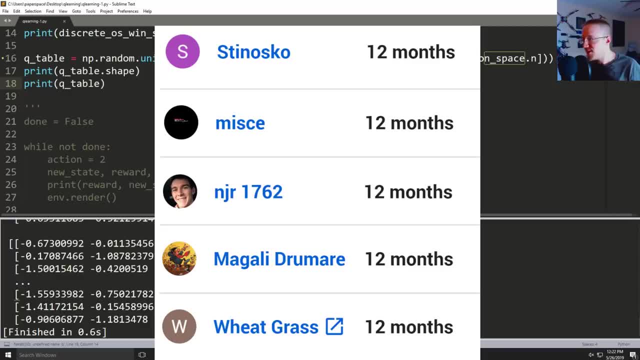 my longest term channel members. these are my longest term channel members. these are people who have been with me. people who have been with me, people who have been with me for uh a year or more. that's incredible. for uh a year or more. that's incredible. for uh a year or more. that's incredible. i can't believe it's been a year that. 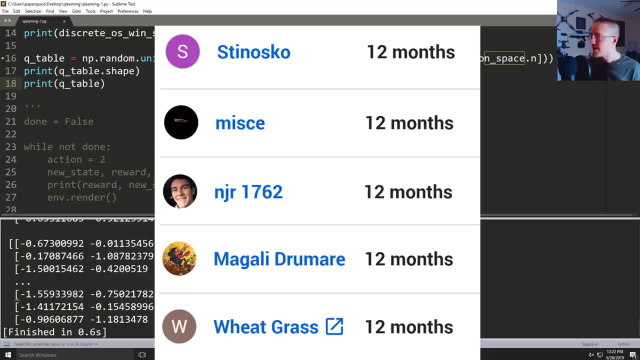 i can't believe it's been a year that. i can't believe it's been a year that i've had these but uh, stenosco. or i've had these, but uh, stenosco. or i've had these but uh, stenosco or stenosco. uh, my longest term member, thank. 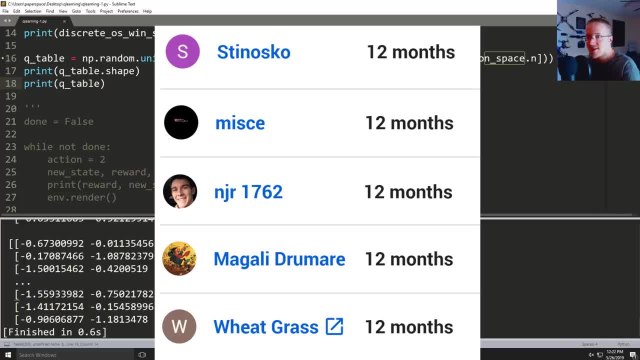 stenosco uh, my longest term member. thank stenosco uh, my longest term member. thank you very much. you're an awesome human. you're an awesome human human being. uh misc njr magali and wheatgrass being. uh misc njr magali and wheatgrass. 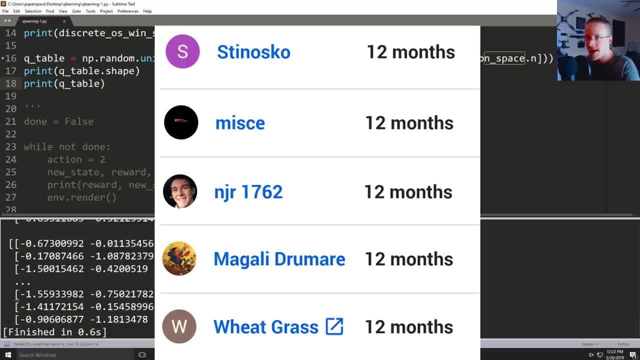 being uh, misc, njr, magali and wheatgrass. thank you all so much for your long-term. thank you all so much for your long-term. thank you all so much for your long-term support. you guys are awesome support. you guys are awesome support. you guys are awesome and you're not just supporting me, you're. 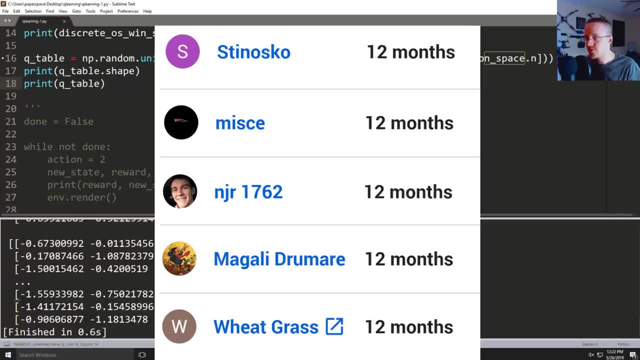 and you're not just supporting me, you're, and you're not just supporting me, you're supporting, supporting, supporting the free education for people who may not, the free education for people who may not, the free education for people who may not be able to afford it otherwise. so 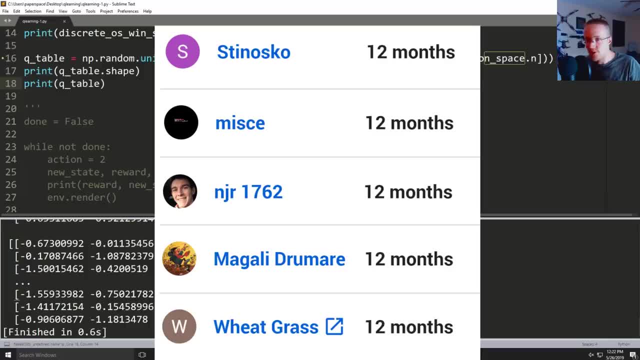 be able to afford it otherwise. so be able to afford it otherwise. so that's really cool. you guys are amazing. that's really cool. you guys are amazing. that's really cool. you guys are amazing people. thank you so much for your people. thank you so much for your. 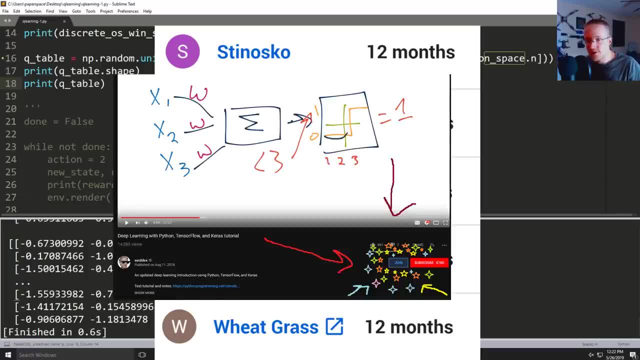 people. thank you so much for your support. if you guys want to support the support, if you guys want to support the support, if you guys want to support the channel, you can click on that blue channel. you can click on that blue channel. you can click on that blue join button. i know some people don't. 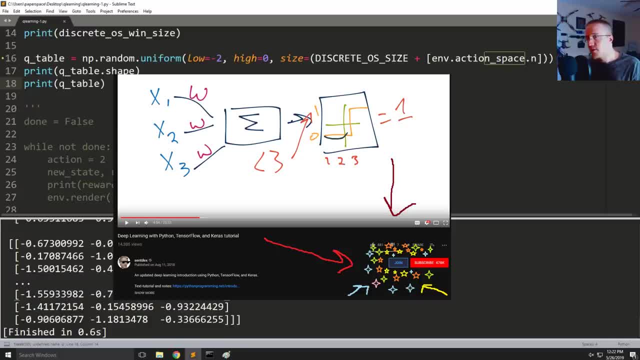 join button. i know some people don't join button. i know some people don't have access to it for some reason, but have access to it for some reason, but have access to it for some reason. but, um, if you have it and you want to, um, if you have it and you want to. 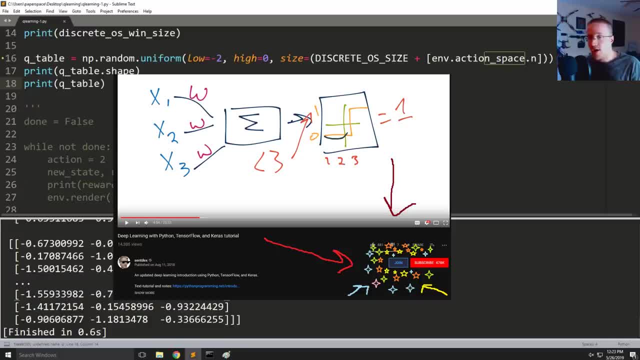 um, if you have it and you want to support the channel, you can click on support the channel. you can click on support the channel. you can click on that right there, that right there, that right there. uh, otherwise, if you've got questions, uh, otherwise, if you've got questions, 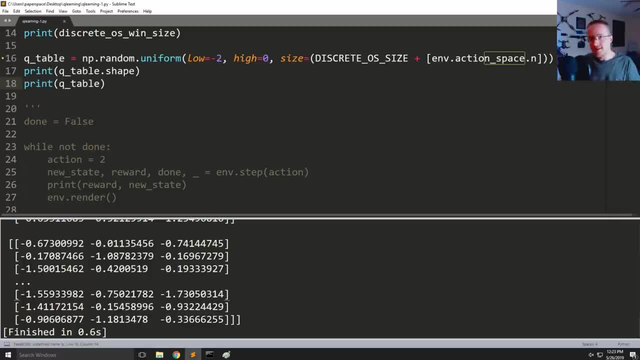 uh, otherwise, if you've got questions, comments whatever about q learning. please comments whatever about q learning. please comments whatever about q learning. please ask them below, ask them below, ask them below. i can't tell you how many q learning. i can't tell you how many q learning. 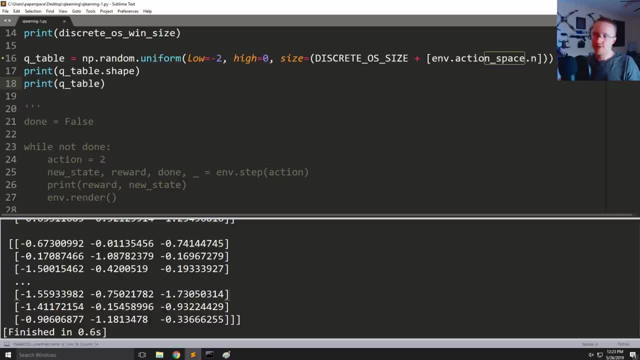 i can't tell you how many q learning tutorials i ended up having to go tutorials. i ended up having to go tutorials. i ended up having to go through before, through, before, through, before slowly figuring it out and um, slowly figuring it out and um, slowly figuring it out and um, i just can't. i hope that. 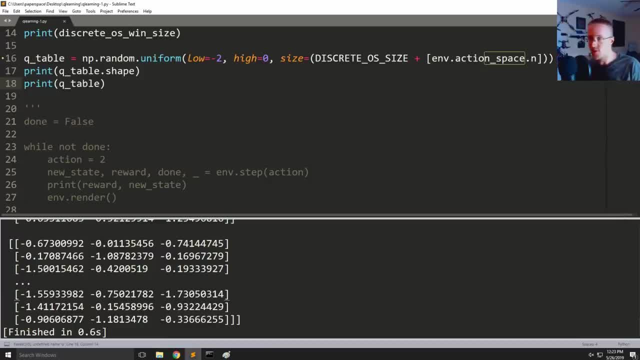 i just can't. i hope that i just can't. i hope that my tutorial will be uh more useful than my tutorial will be uh more useful than my tutorial will be uh more useful than all the other ones that i found myself, all the other ones that i found myself. 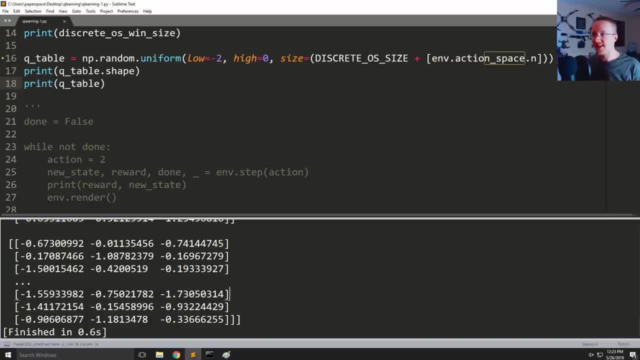 all the other ones that i found myself on so. so if you find yourself lost or on so, so if you find yourself lost or on so, so if you find yourself lost or confused, please ask. i definitely want to confused, please ask. i definitely want to confused. please ask. i definitely want to help you understand q learning. i think. 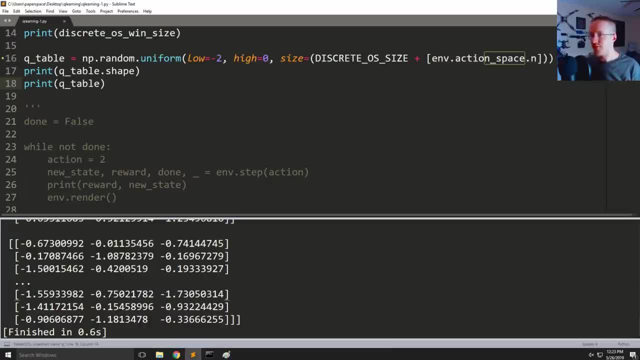 help you understand q learning. i think help you understand q learning. i think it's pretty cool. so anyway, in the next it's pretty cool. so anyway, in the next it's pretty cool. so anyway, in the next video we will hopefully finish up our video, we will hopefully finish up our. 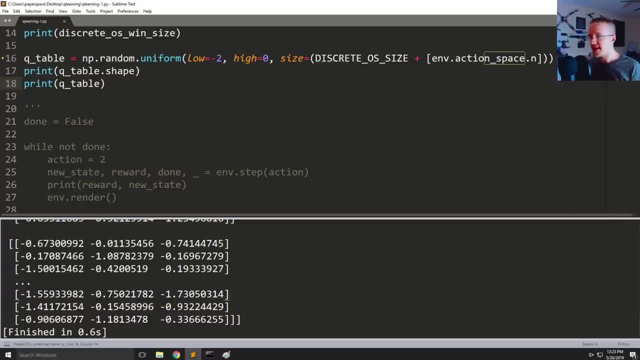 video we will hopefully finish up. our agent actually have it. agent actually have it. agent actually have it driving on to that flag, every single driving on to that flag, every single driving on to that flag, every single time, time, time. uh, anyway, i will see you guys. uh, anyway, i will see you guys.